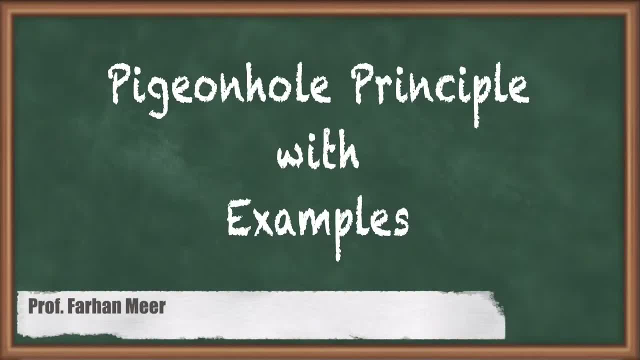 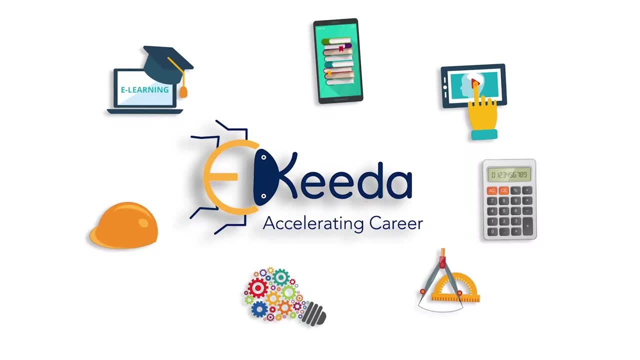 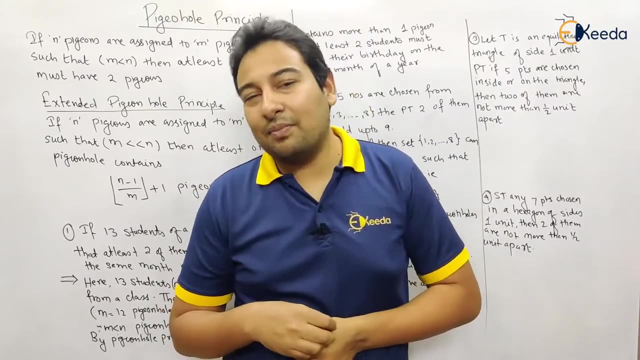 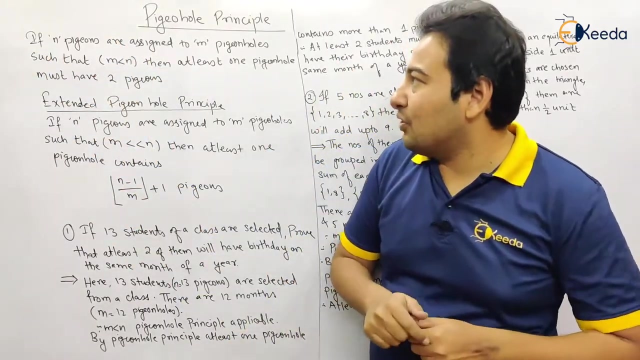 Hello friends, in this video we will talk about Pigeonhole Principle with examples. Welcome back, friends. Let's discuss Pigeonhole Principle, a very simple principle yet very important. So let's read the definition first. If n pigeons are assigned to m pigeonholes. 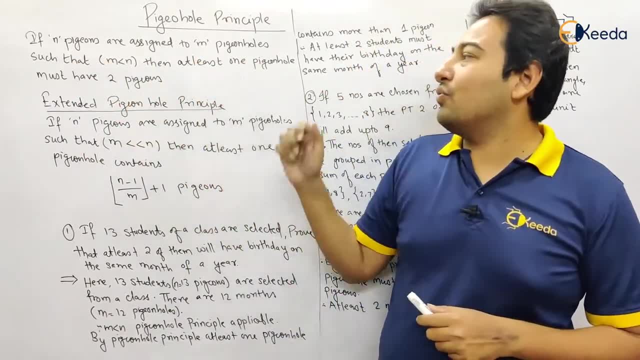 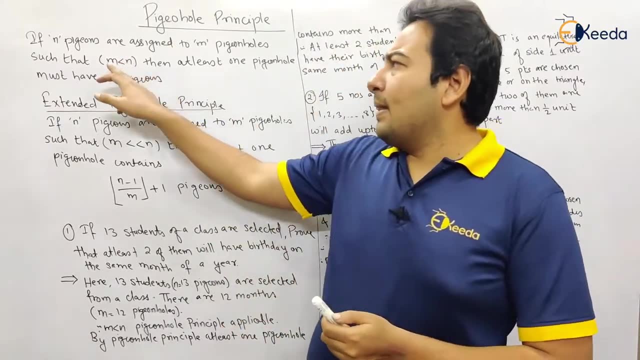 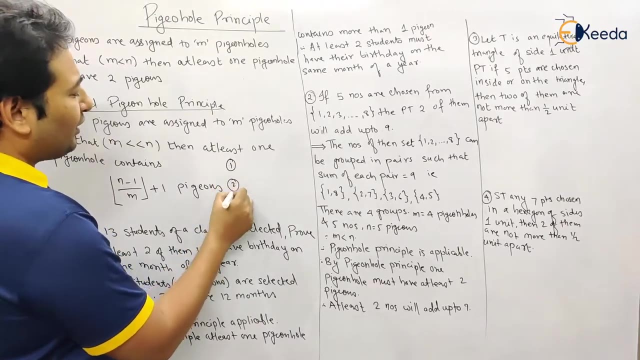 such that m is less than n, then at least one pigeonhole must have two pigeons. So this is the definition of Pigeonhole Principle where the condition is m must be less than n. Now I will explain you with the help of an example, Very simple principle I am considering. 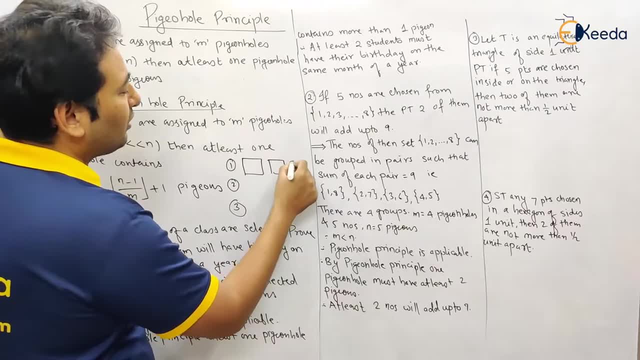 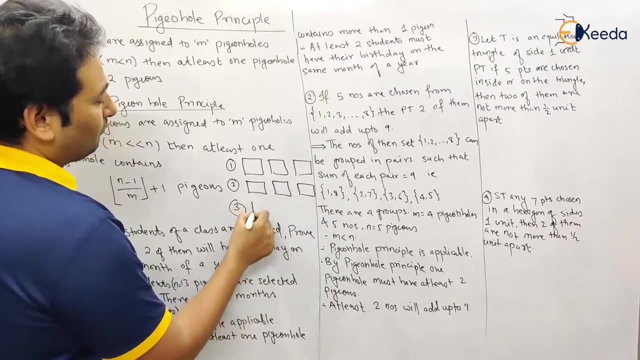 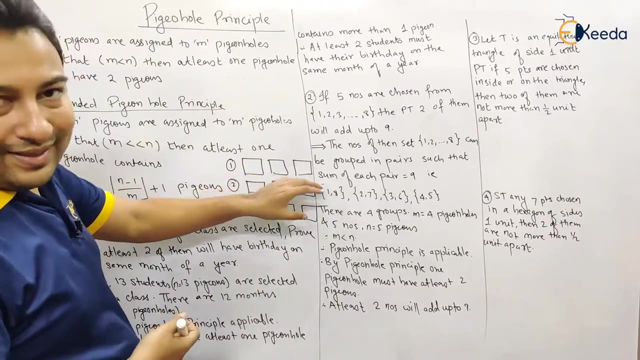 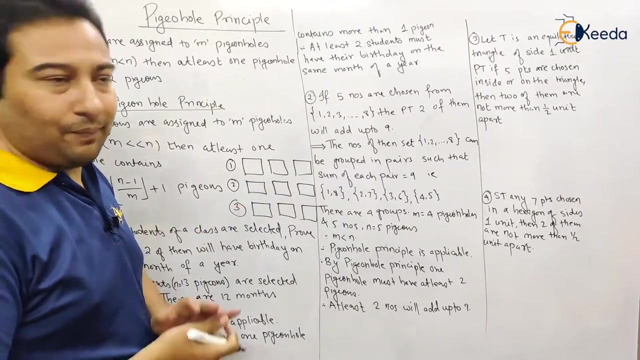 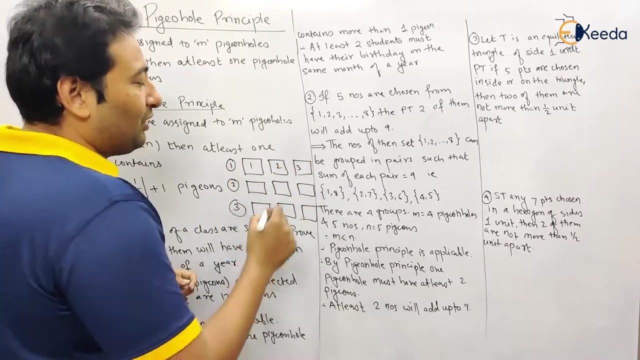 three scenarios here. Suppose these are my pigeonholes. I am considering three pigeonholes and suppose there are four pigeons. Now please tell me how these four pigeons can be assigned to these three pigeonholes. See worst possibility: First pigeon assigned to this pigeonhole. second pigeon, third pigeon, Now fourth pigeon. 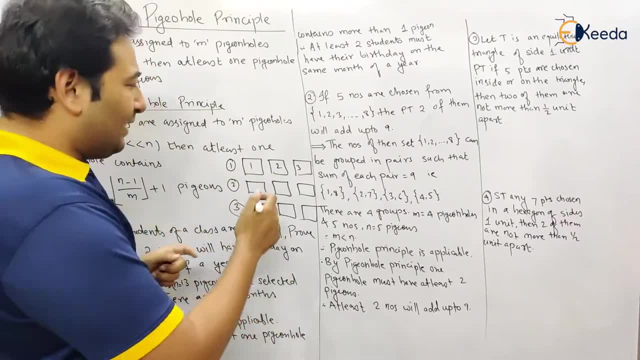 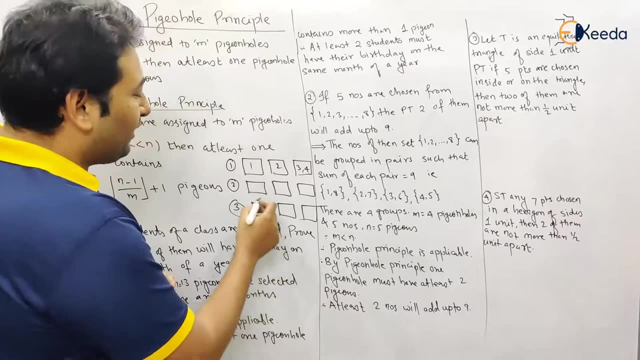 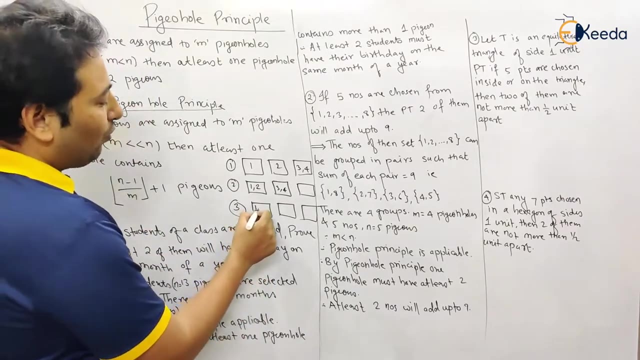 Which pigeonhole will contain the fourth pigeon. Suppose the fourth pigeon is assigned to this particular pigeonhole. What is the next possibility? One, two here, three, four here and the last pigeonhole is empty. What is the next probability? One, two, three, four, all are here. remaining two are 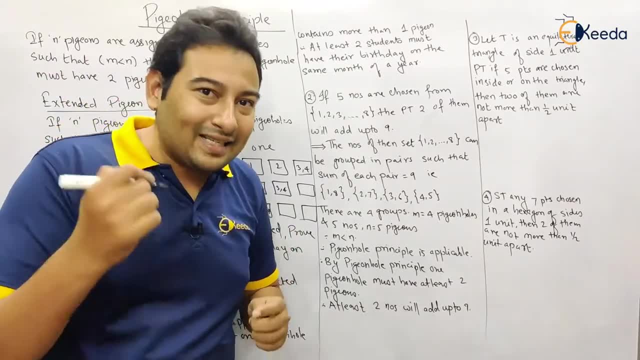 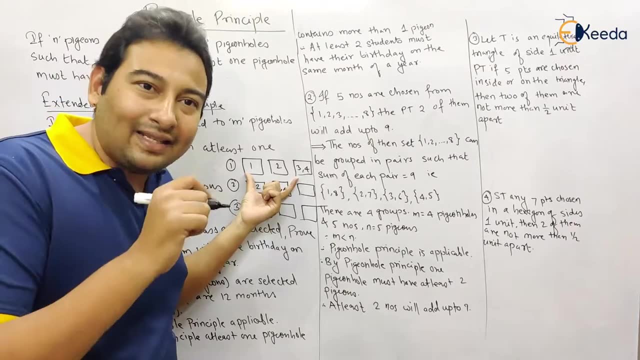 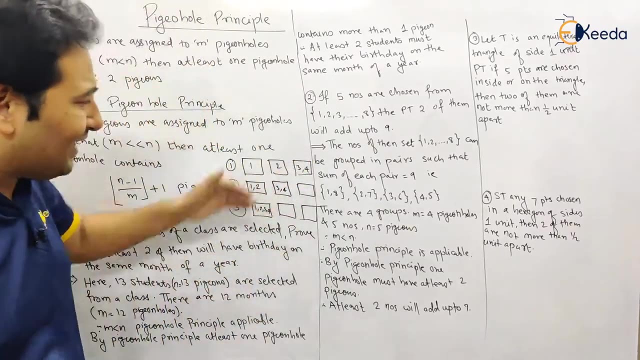 empty. So there are a number of possibilities. My point is: if see how many pigeons are there Four And how many pigeonholes are there Three. So pigeonholes are less, pigeons are more. So the definition says at least one pigeonhole have two pigeons. So check any condition, See. 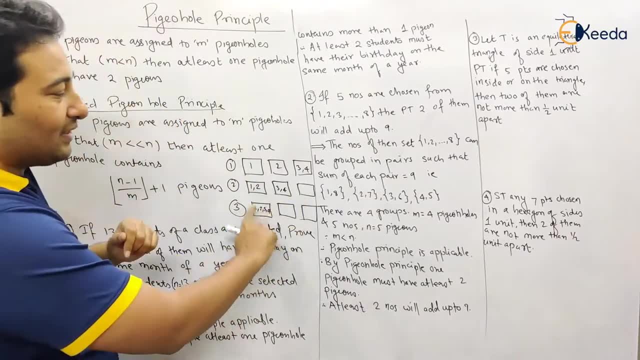 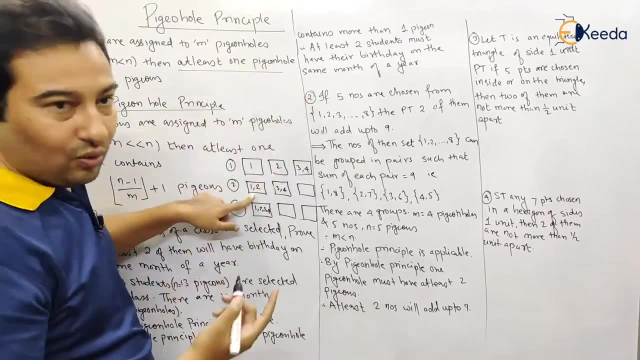 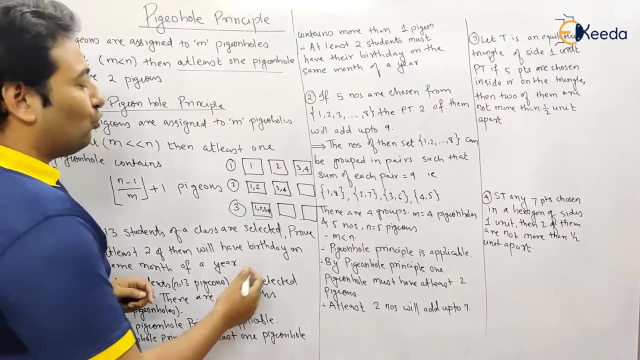 at least one pigeonhole must contain two pigeons. At least one. See, it's not containing any pigeon. This is also containing two, But the criteria is at least one pigeonhole. So at least one pigeonhole must contain two pigeons. At least one pigeonhole contains two pigeons. These are: 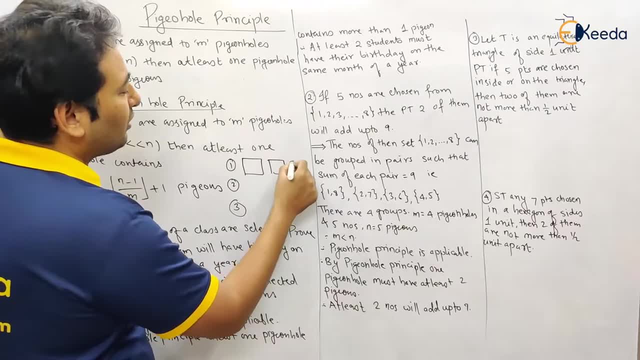 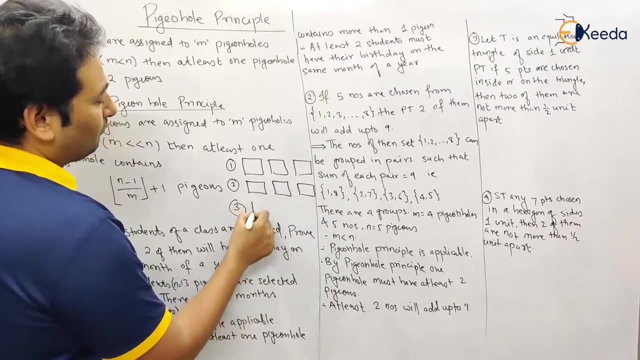 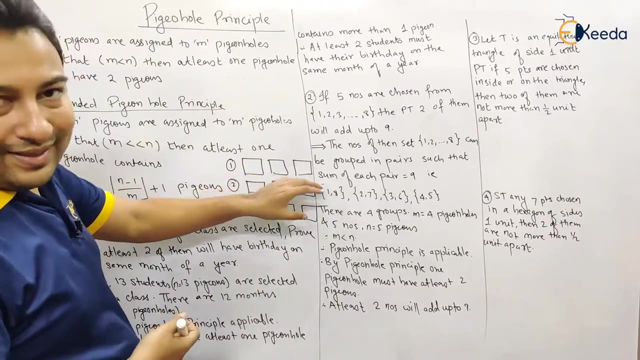 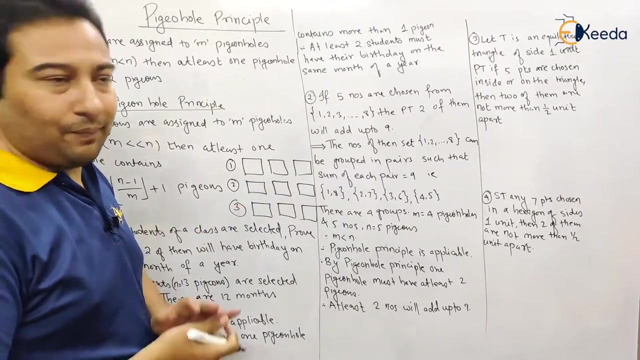 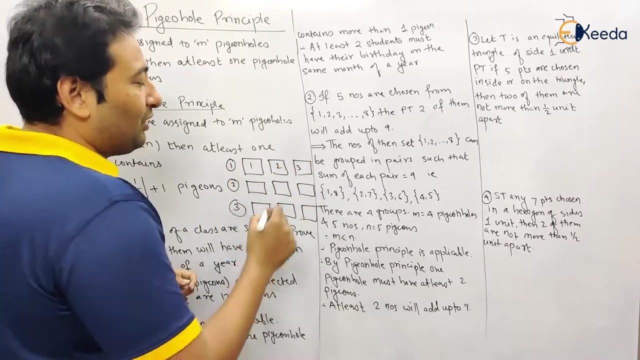 three scenarios here. Suppose these are my pigeonholes. I am considering three pigeonholes and suppose there are four pigeons. Now please tell me how these four pigeons can be assigned to these three pigeonholes. See worst possibility: First pigeon assigned to this pigeonhole. second pigeon, third pigeon, Now fourth pigeon. 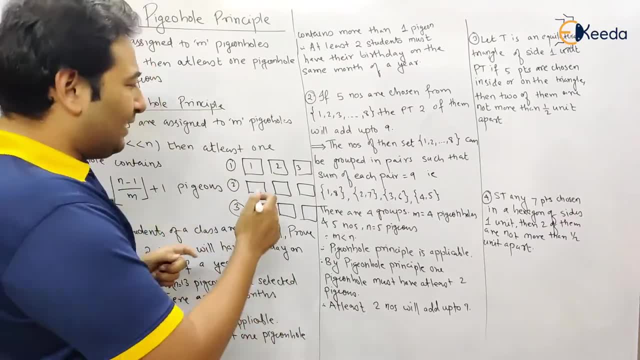 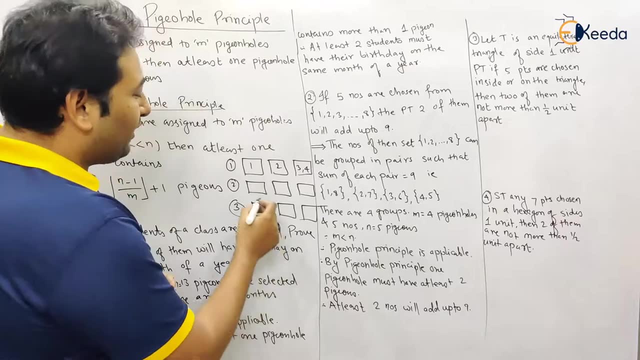 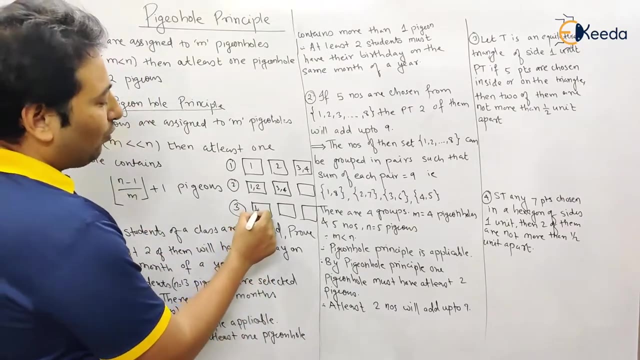 Which pigeonhole will contain the fourth pigeon. Suppose the fourth pigeon is assigned to this particular pigeonhole. What is the next possibility? One, two here, three, four here and the last pigeonhole is empty. What is the next probability? One, two, three, four, all are here, remaining two. 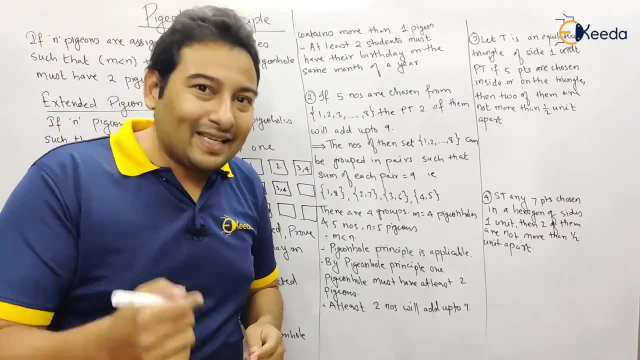 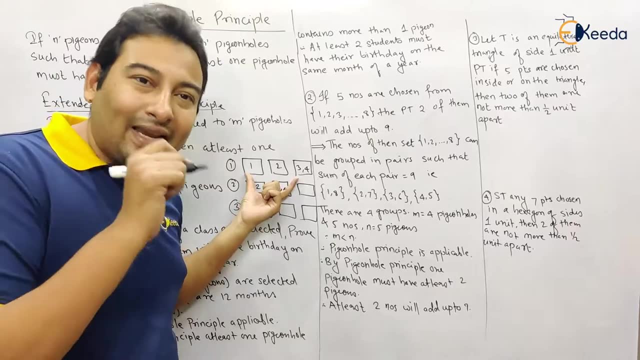 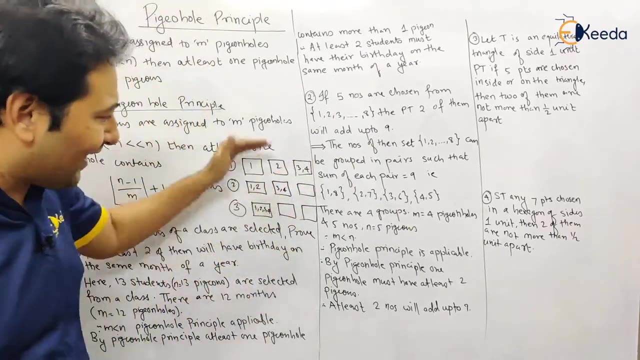 are empty. So there are a number of possibilities. My point is: if see how many pigeons are there Four And how many pigeonholes are there Three. So pigeonholes are less, pigeons are more. So the definition says at least one pigeonhole have two pigeons. So check any condition, See. 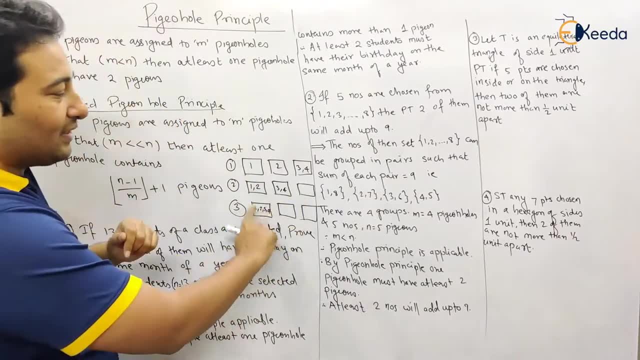 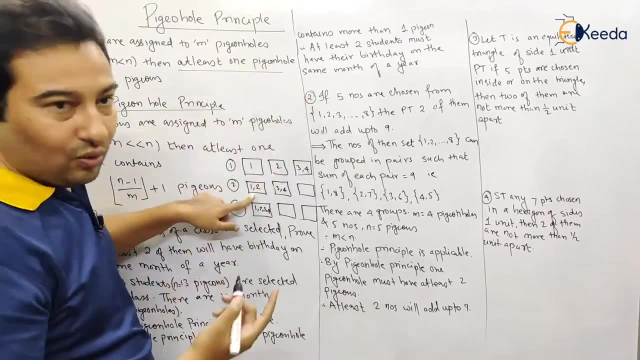 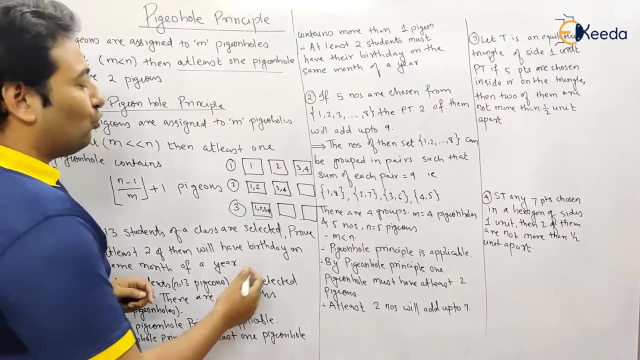 at least one pigeonhole must contain two pigeons. At least one. See, it's not containing any pigeon. This is also containing two, But the criteria is at least one pigeonhole. So at least one pigeonhole must contain two pigeons. At least one pigeonhole contains two pigeons. These are: 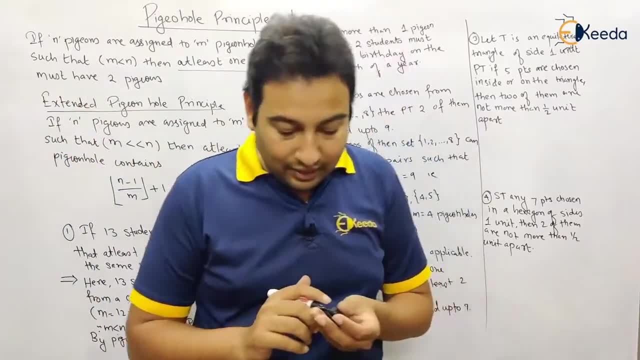 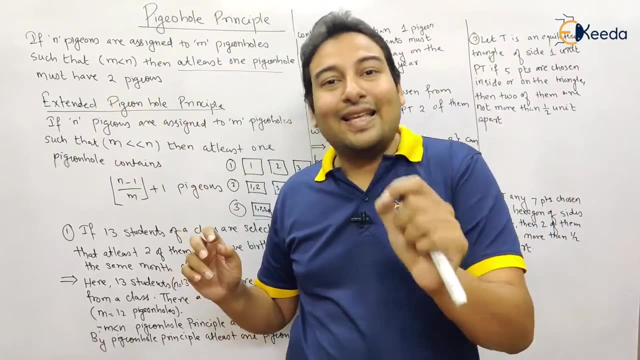 empty Doesn't matter. So is this point clear? Is this definition clear? So what is the definition? If there are n pigeons, m pigeonholes- Condition is pigeonholes are less than pigeons- Then there is at least one pigeonhole which contains two pigeons. So this is the definition. 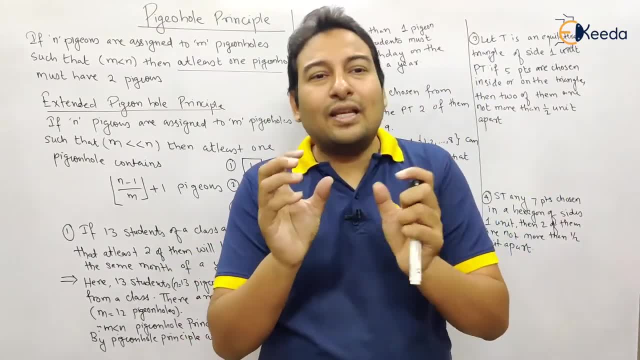 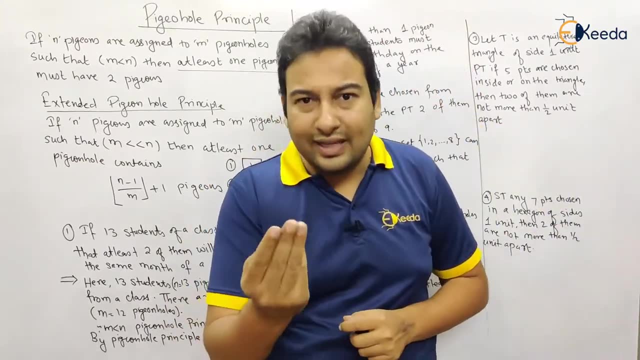 of pigeonhole principle And when it is used, if there is a very small difference between pigeonhole and pigeons. Likewise, I have given you the example Here- the pigeonholes are three and pigeons are four. So there is a difference of one, So very small difference, one, two difference. 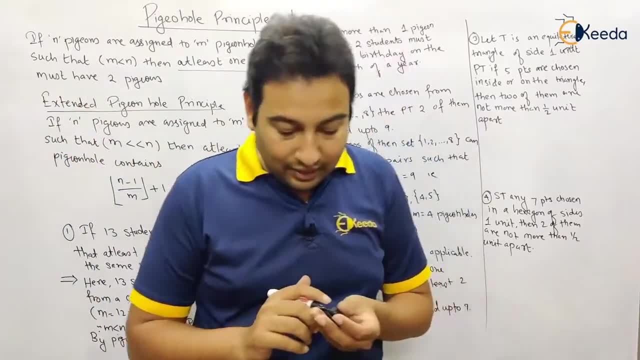 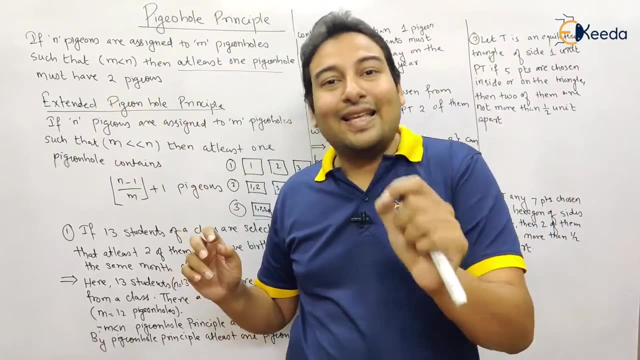 empty Doesn't matter. So is this point clear? Is this definition clear? So what is the definition? If there are n pigeons, m pigeonholes- Condition is pigeonholes are less than pigeons- Then there is at least one pigeonhole which contains two pigeons. So this is the definition. 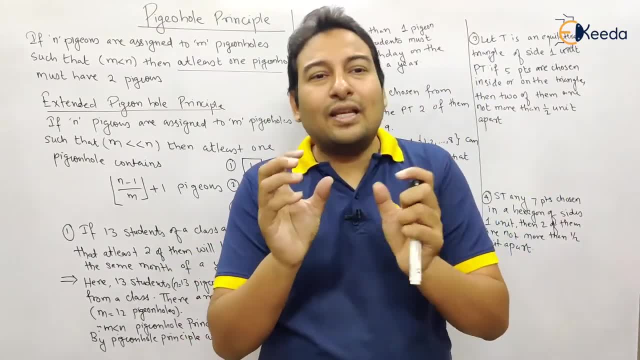 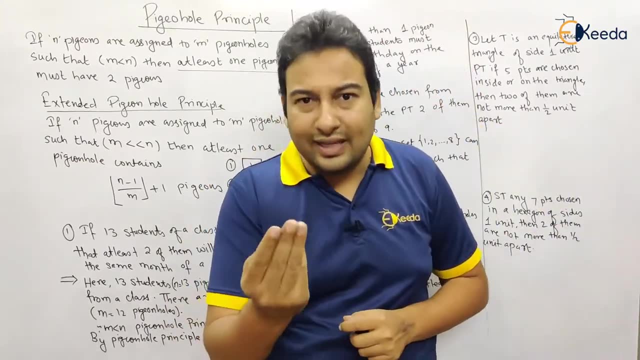 of pigeonhole principle And when it is used, if there is a very small difference between pigeonhole and pigeons. Likewise, I have given you the example Here- the pigeonholes are three and pigeons are four. So there is a difference of one, So very small difference, one, two difference. 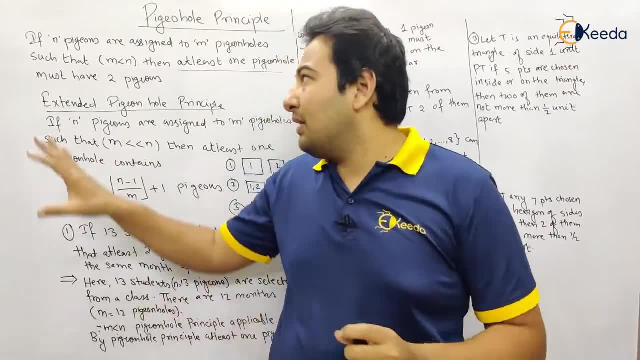 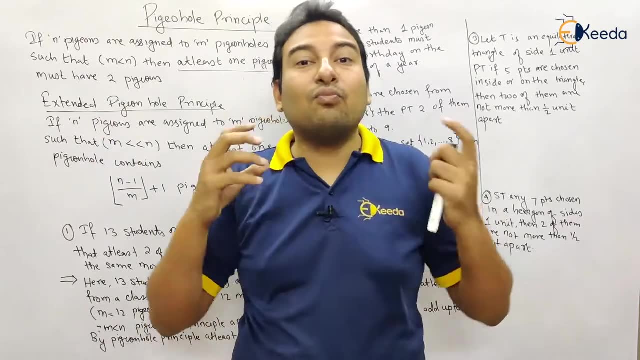 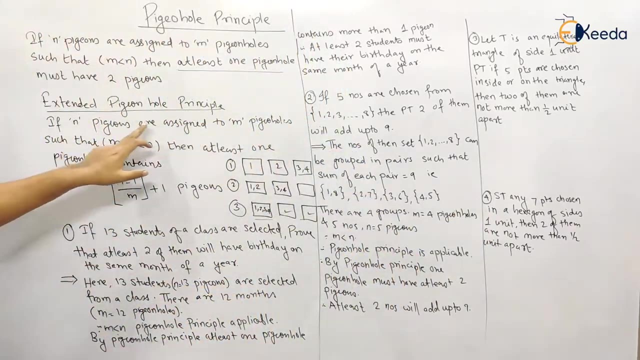 If there is a very small difference between the pigeons and the pigeonhole principle, then we go with the pigeonhole principle, And if there is the difference is more, then we go with extended pigeonhole principle. Again, the concept is same. If n pigeons are assigned to m pigeonholes and 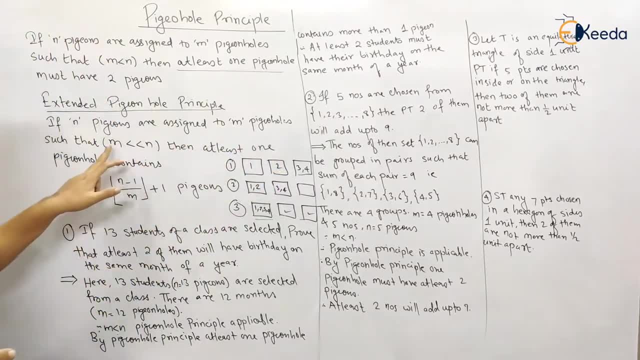 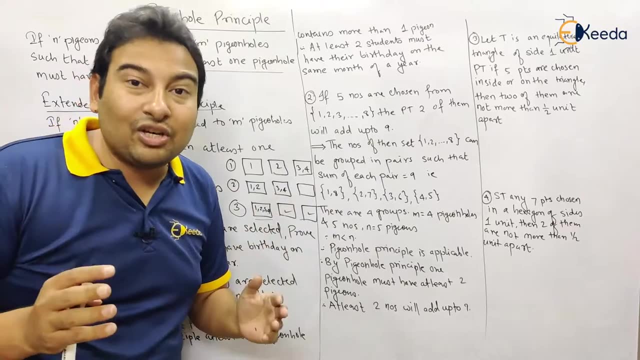 obviously m is less than n, So m is actually very less than n. That means here: suppose there are three pigeons and let's say 100.. Suppose there are three pigeonholes and let's say 100 pigeons. So the difference is more. Are you getting my point? 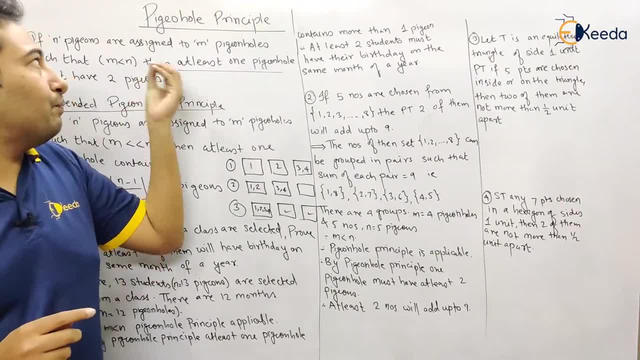 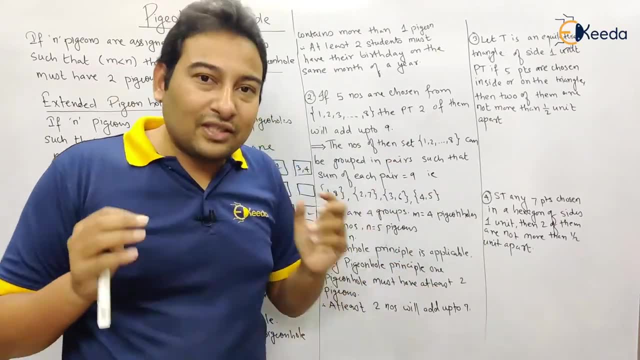 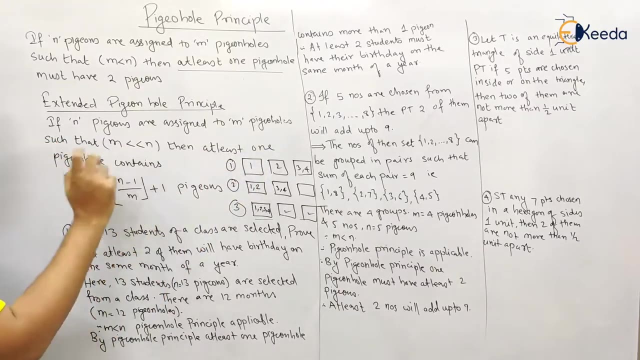 Three pigeonholes, four pigeons- You can simply apply pigeonhole principle. But if the difference is more- three pigeonholes, 100 pigeons, So see the difference. If difference is more, then in that case we're going to apply extended pigeonhole principle which says at least one of the pigeonhole. 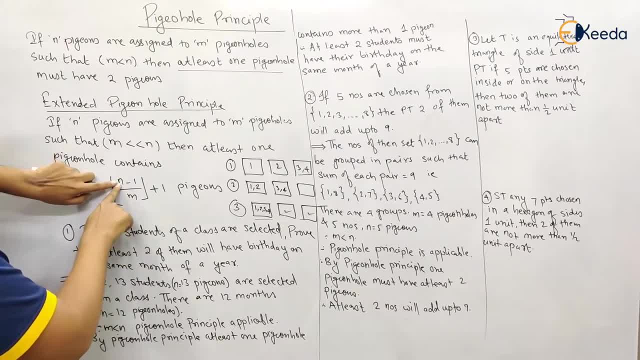 contains this many pigeons, Where n is your number of pigeons, m is number of pigeonholes plus one pigeons, And this is what your floor function. This is what we discussed in set theory, also in principle of inclusion, exclusion. So what do you mean by floor function? 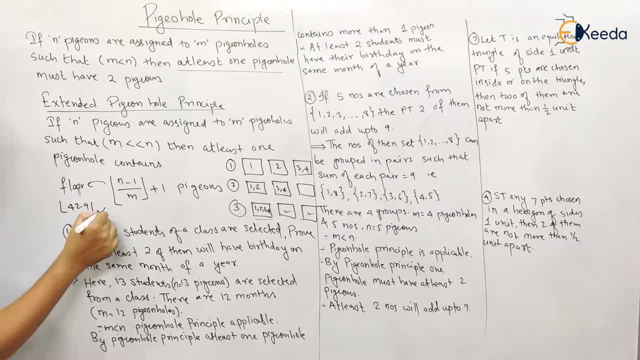 Floor function means if you get 42.9, still it will take 42. So it is going to consider the lowest integer. So 42.9 means 42.. 42.1 also means 42. See 42.9 is lying between 42 and 43. It's going. 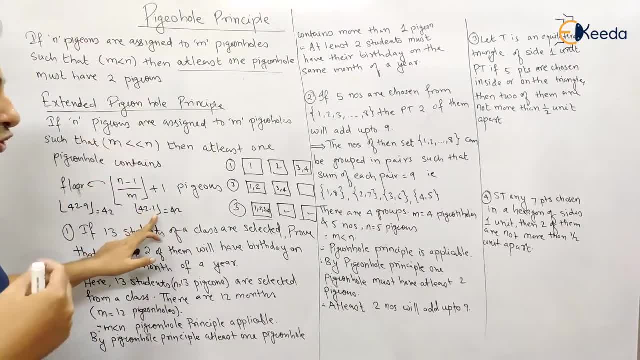 to take the lowest integer, That is 42. Again, 42.1 is lying between 42 and 43. So lowest integer it is going to pick. So this is what pigeonhole and extended pigeonhole principle. So in this video we'll talk about pigeonhole principle examples. In the next 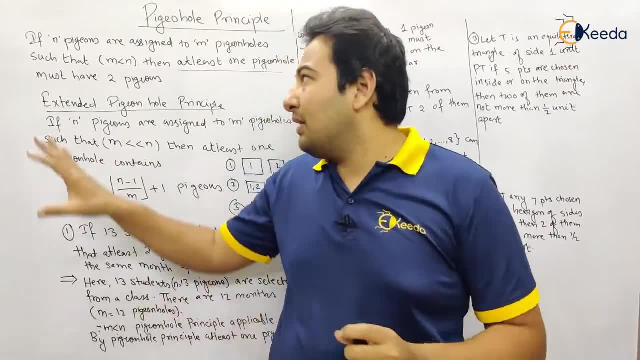 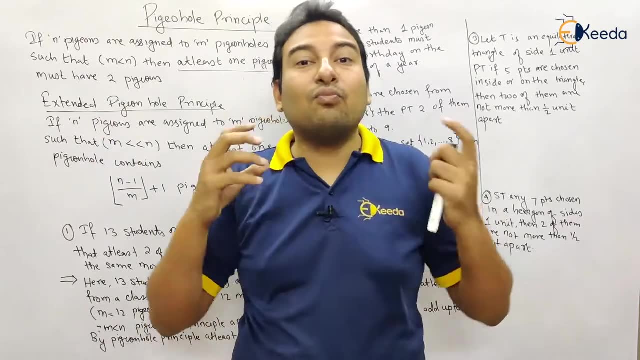 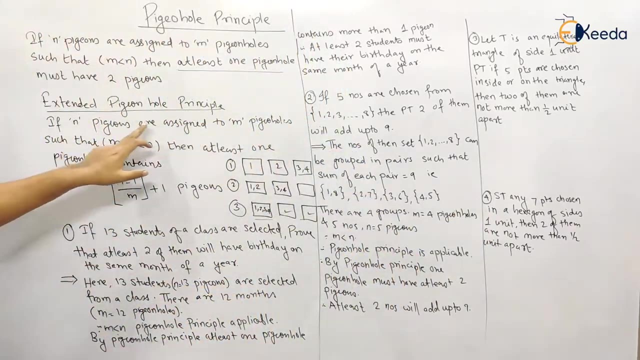 If there is a very small difference between the pigeons and the pigeonhole principle, then we go with the pigeonhole principle, And if there is the difference is more, then we go with extended pigeonhole principle. Again, the concept is same. If n pigeons are assigned to m pigeonholes and 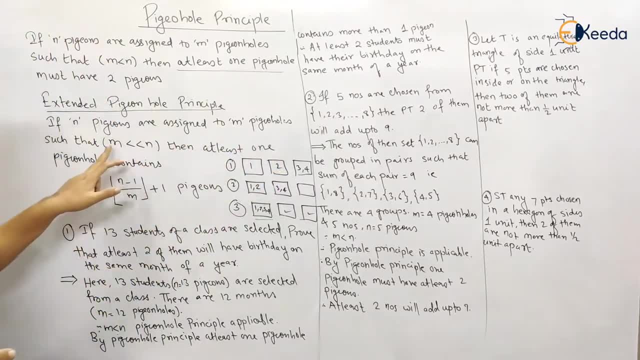 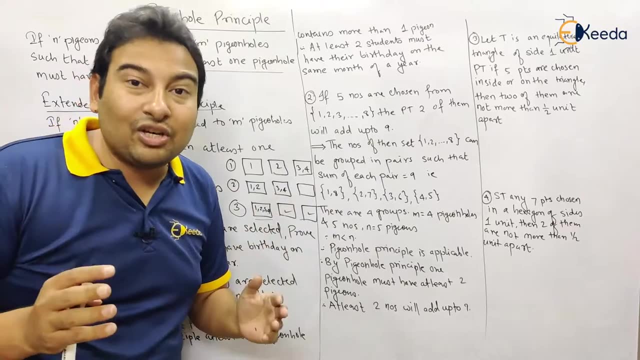 obviously m is less than n, So m is actually very less than n. That means here: suppose there are three pigeons and let's say 100.. Suppose there are three pigeonholes and let's say 100 pigeons. So the difference is more. Are you getting my point? 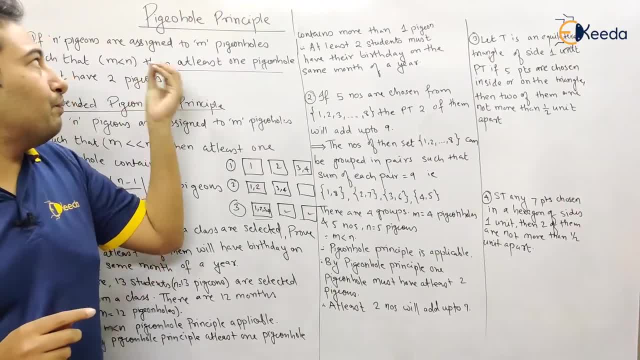 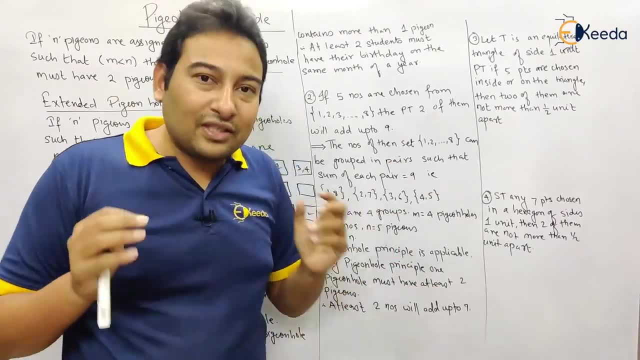 Three pigeonholes, four pigeons- You can simply apply pigeonhole principle. But if the difference is more- three pigeonholes, 100 pigeons, So see the difference. If difference is more, then in that case we're going to apply extended pigeonhole principle which says at least one of the 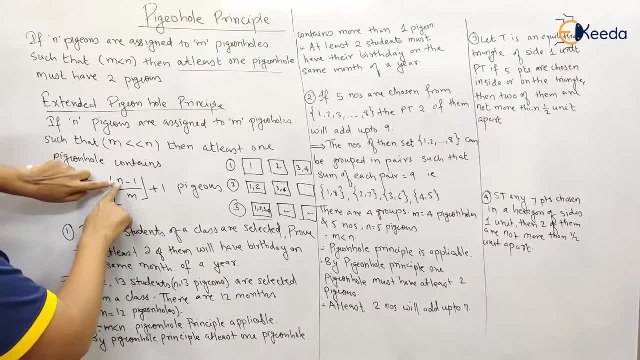 pigeonhole contains this many pigeons. Where n is your number of pigeons? m is number of pigeonholes plus one pigeons, And this is what your floor function. This is what we discussed in set theory, also in principle of inclusion-exclusion. So what do you mean by floor function? Floor. 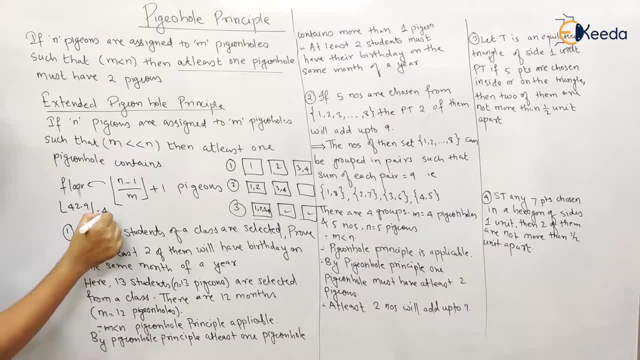 function means: if you get 42.9, still it will take 42. So it is going to consider the lowest integer. So 42.9 means 42.. 42.1 also means 42. See: 42.9 is lying between 42 and 43. It's going. 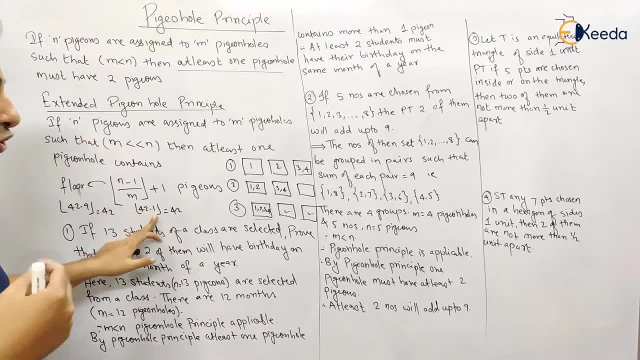 to take the lowest integer, That is 42. Again, 42.1 is lying between 42 and 43. So lowest integer it is going to pick. So this is what pigeonhole and extended pigeonhole principle. So in this video we'll talk about pigeonhole principle examples. In the next 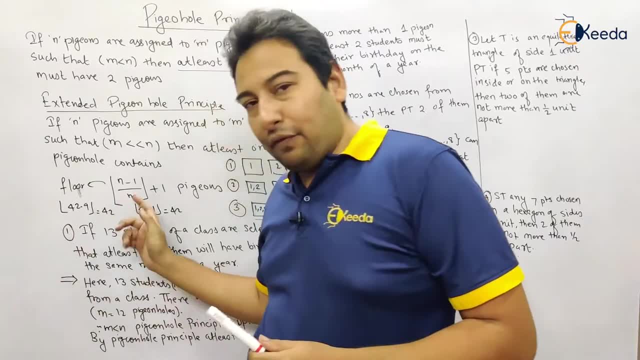 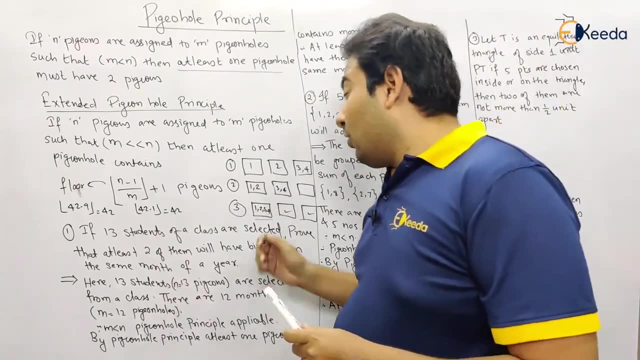 video. we'll talk about extended pigeonhole principle examples. So the first problem: 13 students of class are selected, Proof that at least two of them will have their birthday on the same month of a year. How many students selected 13.. How many months are there? 12.? 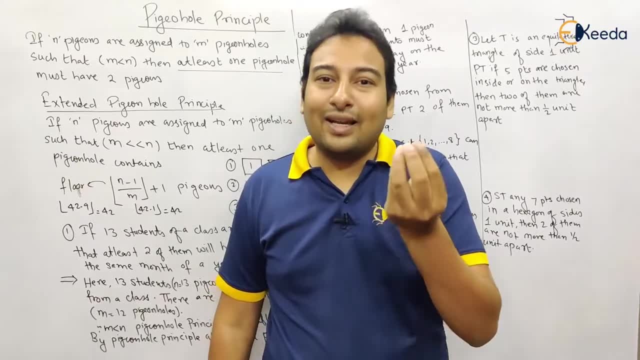 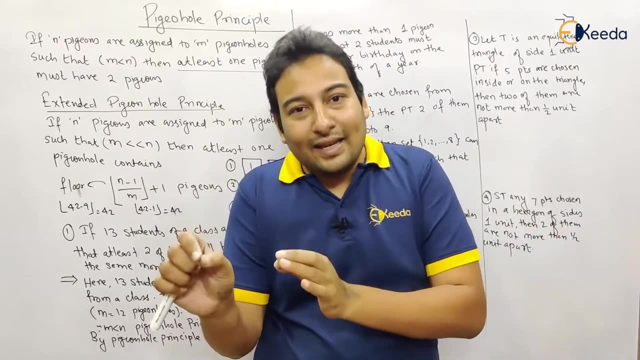 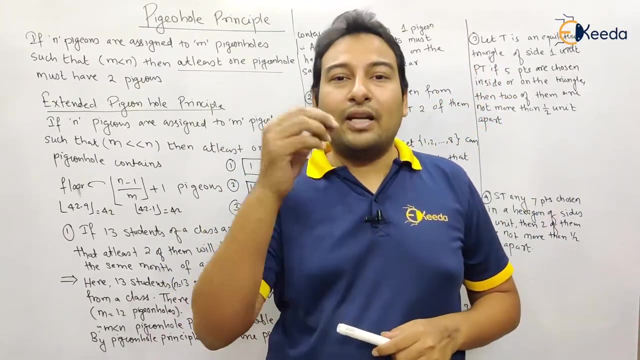 Story over. So 13 students means there are 13 pigeons, and 12 months means 12 pigeonholes. Here m is less than n. Therefore, by pigeonhole principle, at least one of the students, at least two students, will have their. 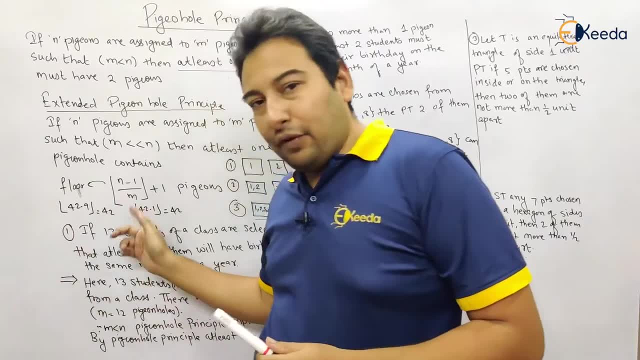 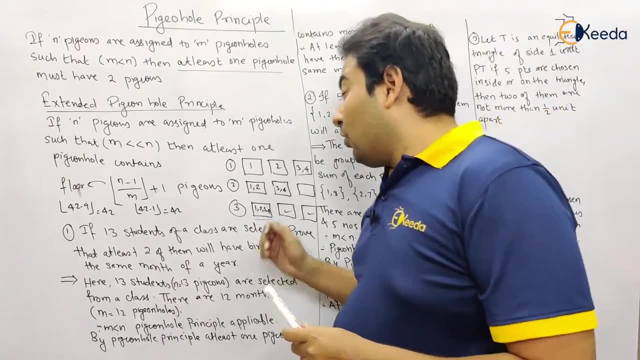 video. we'll talk about extended pigeonhole principle examples. So the first problem: 13 students of class are selected, Proof that at least two of them will have their birthday on the same month of a year. How many students selected 13.. How many months are there? 12.? 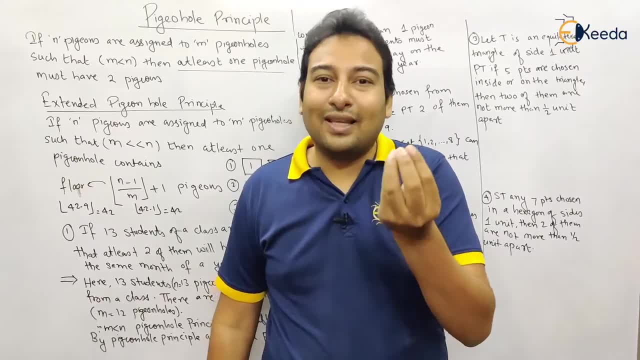 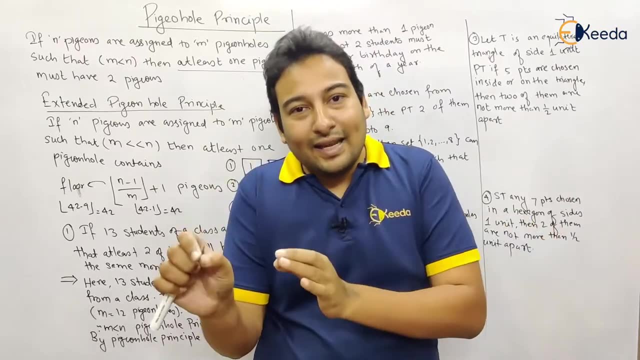 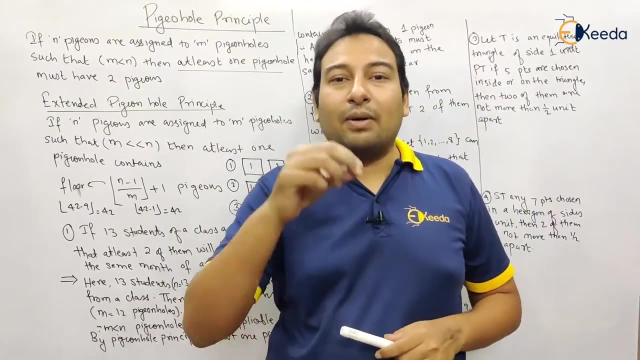 Story over. So 13 students means there are 13 pigeons and 12 months means 12 pigeonholes. Here M is less than N. Therefore, by pigeonhole principle, at least one of the students, at least two students, will have their. 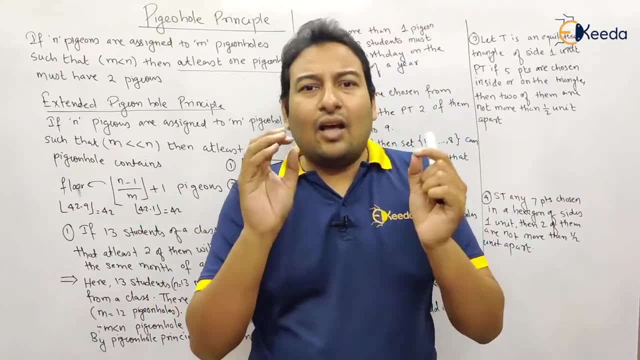 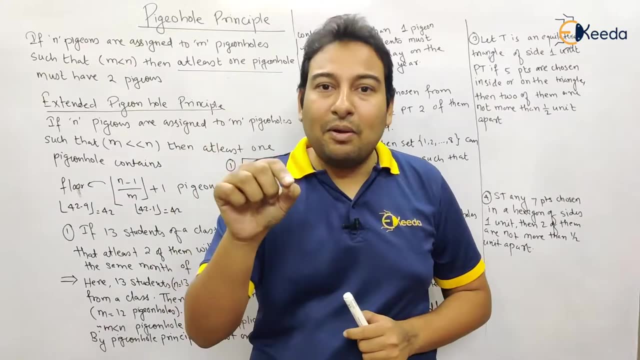 birthday on the same month. See, that's it. It's done. Obviously, if there are 13 students, if all the students are born on different month, at least there will be a month. 13 students will be born in one of the months. That means at least there will be one month in which. 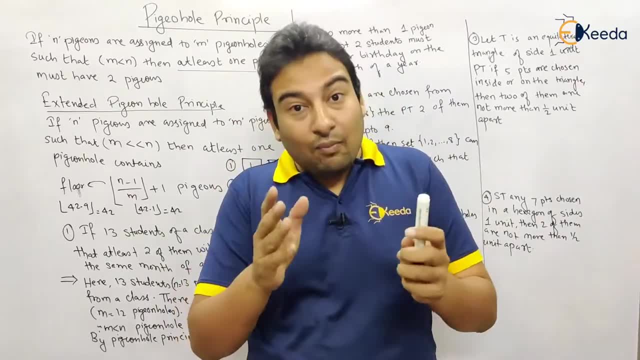 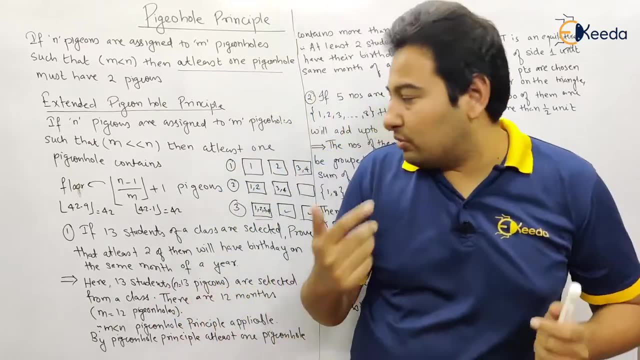 there are two students born, There is a possibility that all the students born on the same month, So at least there is a month in which there are more than two students born. That's it Story over. See the question. If 13 students are selected of a class, proof that at least two of them will have. 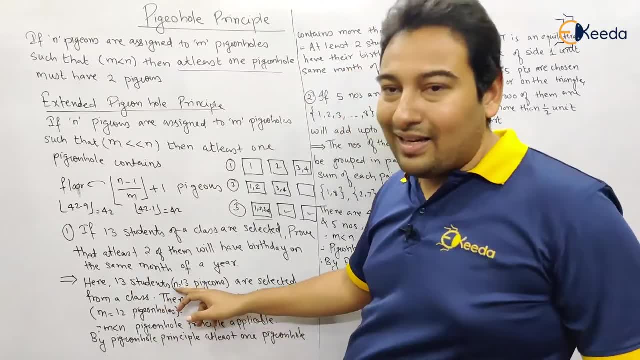 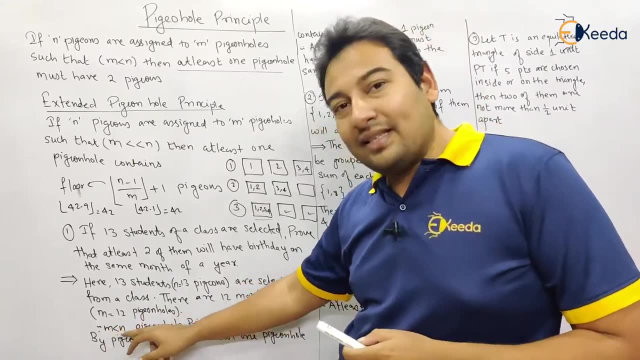 their birthday on the same month of a year. So 13 students mean N is equal to 13,. that is pigeons are selected from a class. There are 12 months, that is M is equal to 12 pigeons. M is less than. 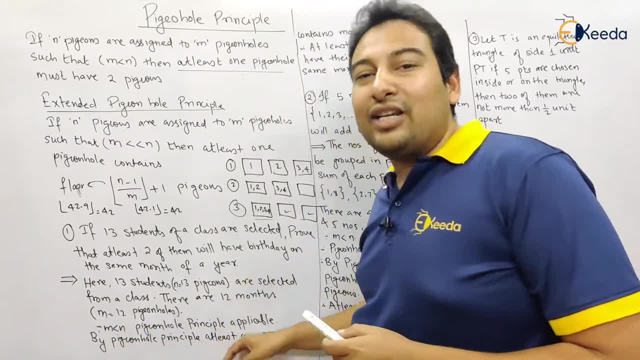 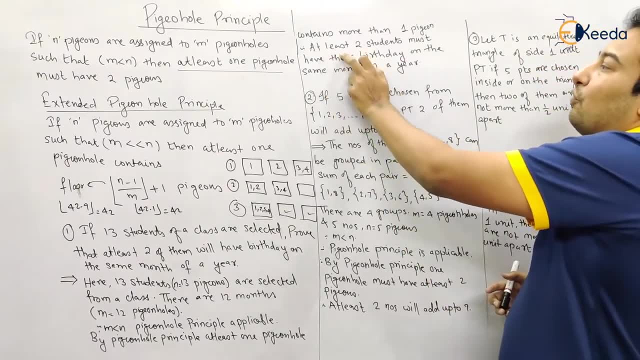 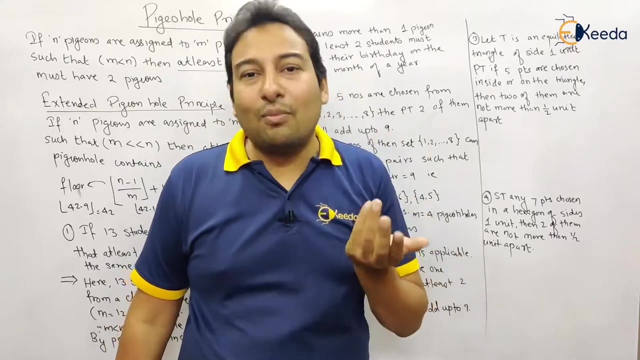 N. Pigeonhole principle is applicable. By pigeonhole principle, at least one pigeonhole must have two pigeons. Therefore, at least two students must have their birthday on the same month of a year. That's it Story over. It's actually a very simple thing. It's just a common sense, Nothing else. Next, 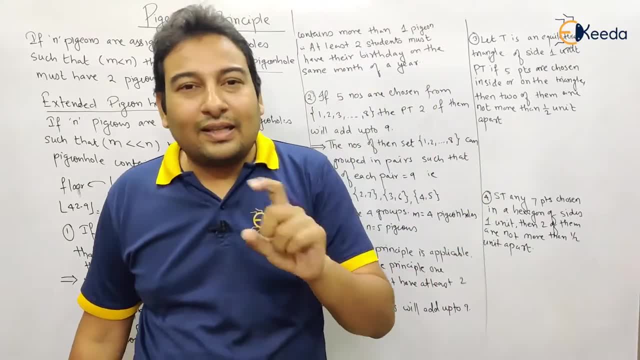 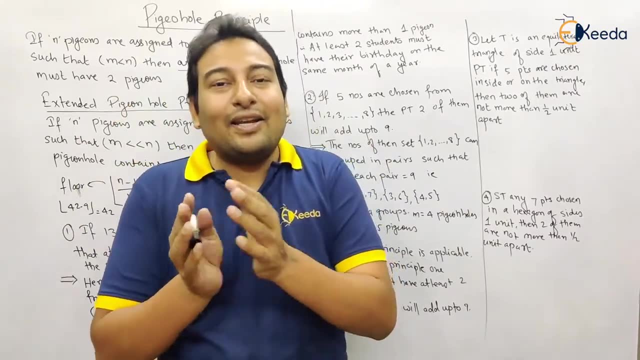 suppose, suppose, suppose. let me give you one more example. There are seven days in a week. How many students? Let's say, there are eight students. So what will be the question? Eight students are selected. How many students are selected. How many students are selected? How many students are selected? 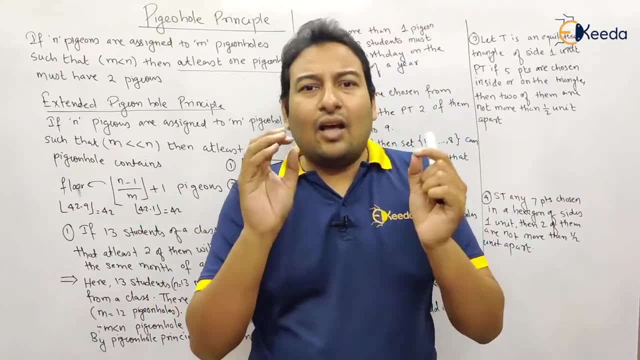 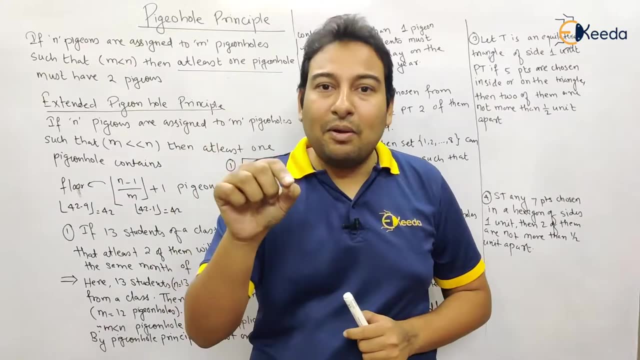 birthday on the same month. See, that's it. It's done. Obviously, if there are 13 students, if all the students are born on different month, at least there will be a month. 13 students will be born in one of the months. That means at least there will be one month in which. 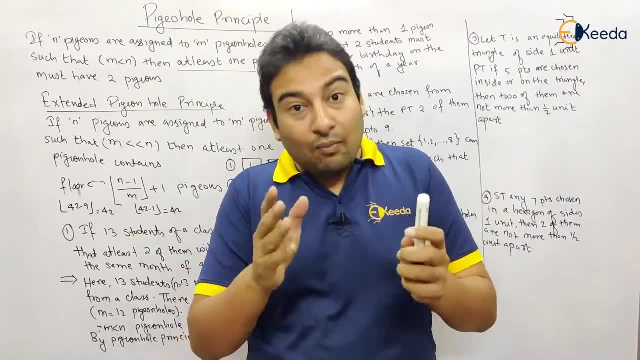 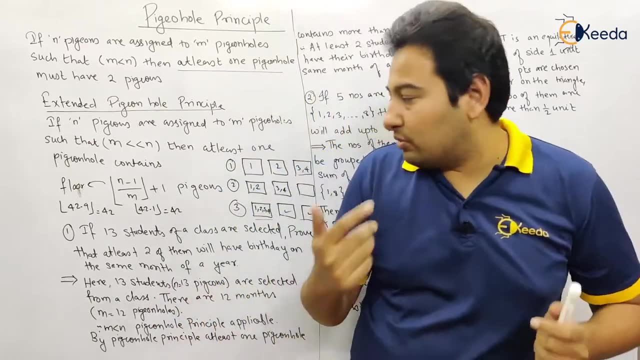 there are two students born, There is a possibility that all the students born on the same month, So at least there is a month in which there are more than two students born. That's it Story over. See the question. If 13 students are selected of a class, proof that at least two of 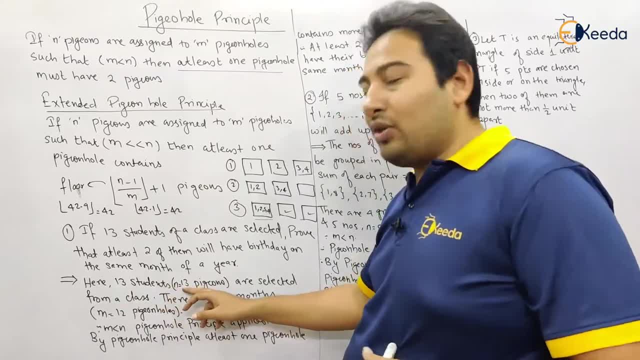 them will have their birthday on the same month of a year. So 13 students mean n is equal to 13,. that is, pigeons are selected from a class. There are 12 months, that is m is equal to 12 pigeons. 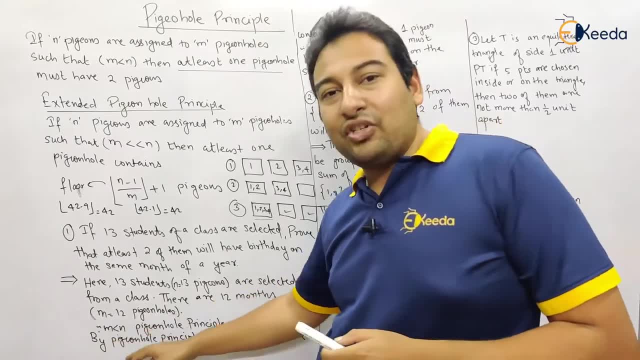 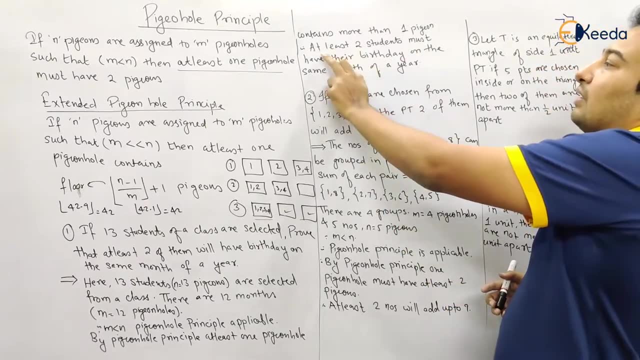 m is less than n. Pigeonhole principle is applicable. By pigeonhole principle, at least one pigeonhole must have two pigeons. Therefore, at least two students must have their birthday on the same month of a year. That's it. 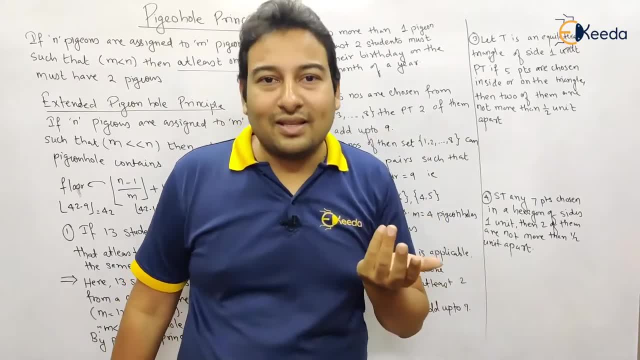 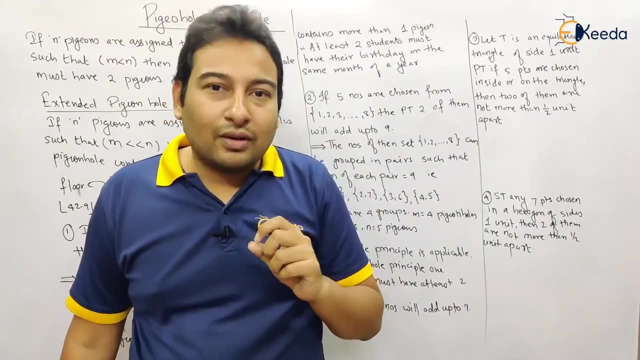 Story over. It's actually a very simple thing, It's just a common sense, Nothing else. Next, suppose, suppose, suppose. let me give you one more example. There are seven days in a week. How many students? Let's say, there are eight students. So what will be the question? 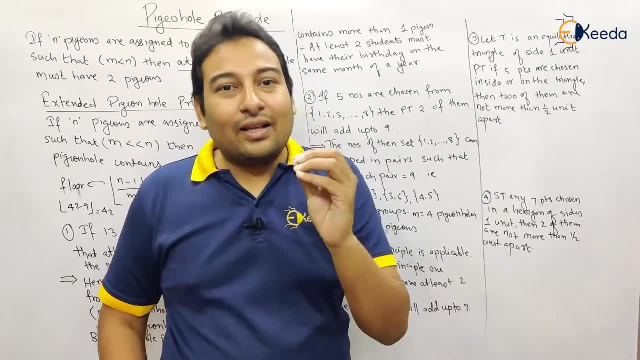 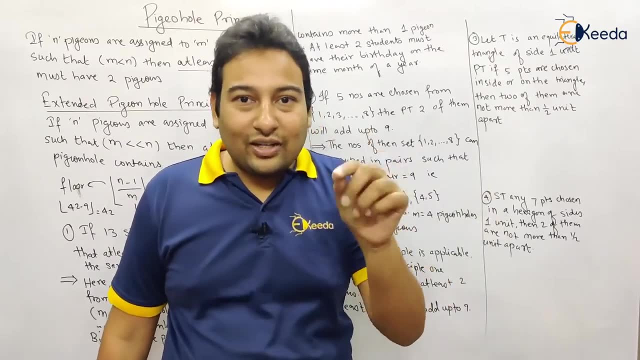 Eight students are selected From a class Prove that at least two of them will have their birthday on the same day of a week. So eight students means what? n is equal to eight pigeons And m is equal to seven, That is. 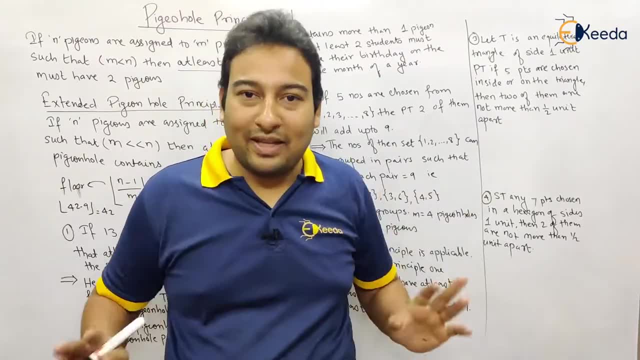 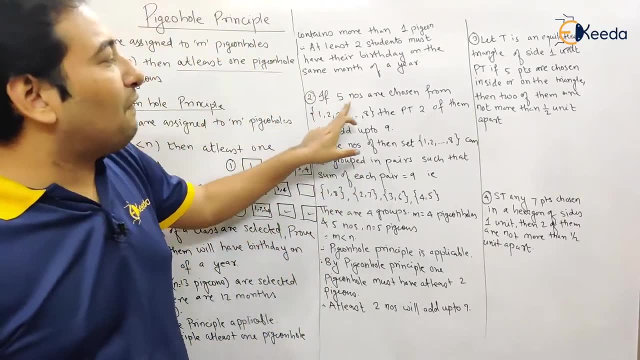 seven pigeonholes. m is less than n, Pigeonhole principle is applicable. That's it Story over. Next question. Now this problem is a very important problem. It is asked a number of times in the exam. If five numbers are chosen from and see, we have written the solution also. 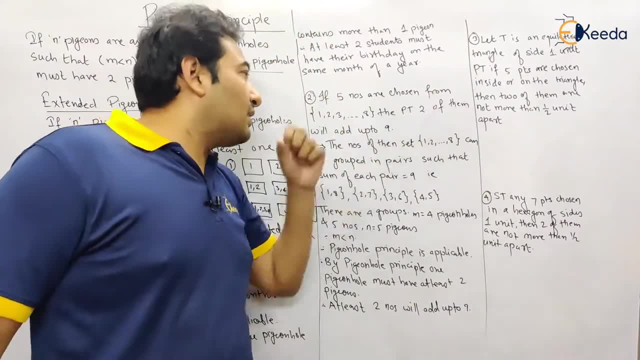 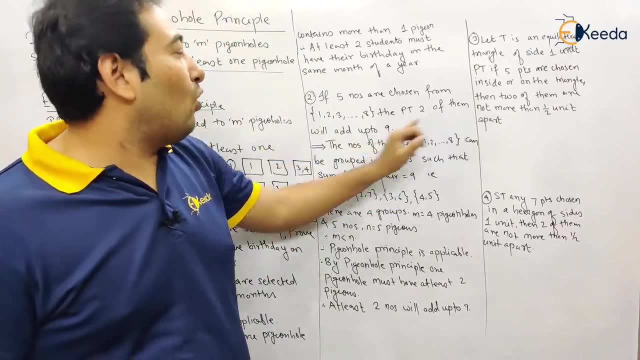 You need to write it down in this particular format. If five numbers are chosen, from one to eight, So between one to eight, five numbers are chosen, We need to prove that two of them will add up to nine. We need to prove that two of them will add up to nine. So you need to remember in this: 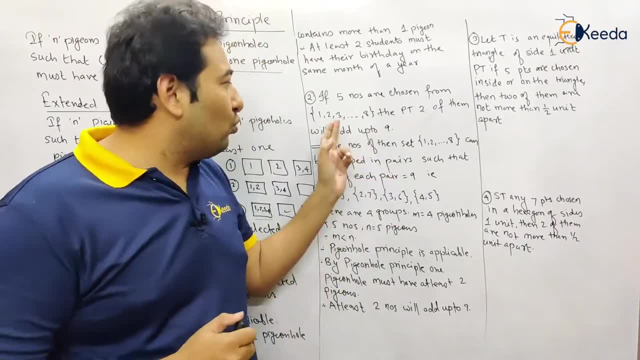 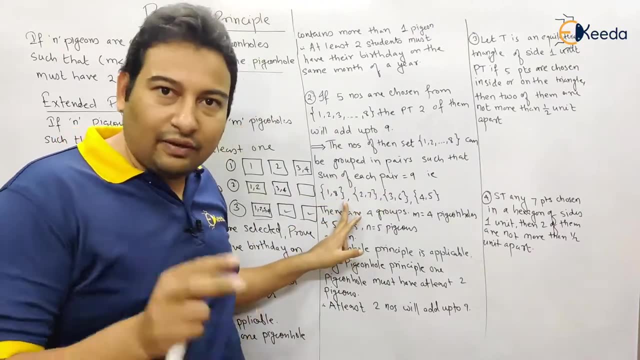 particular problem. See: two of them will add up to nine. So two numbers adding up to nine. So between one to eight, which two numbers will add up to nine? The first pair is 1,8.. That will add up to nine. If you add, you'll get nine. 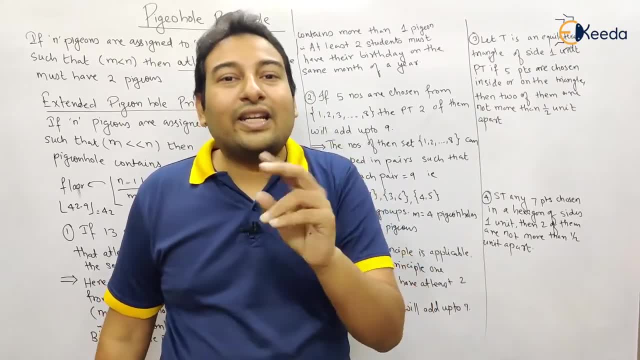 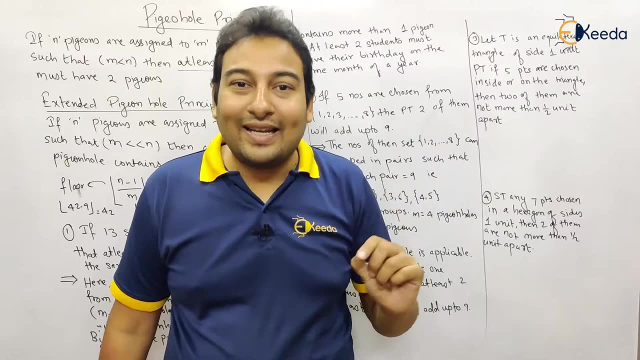 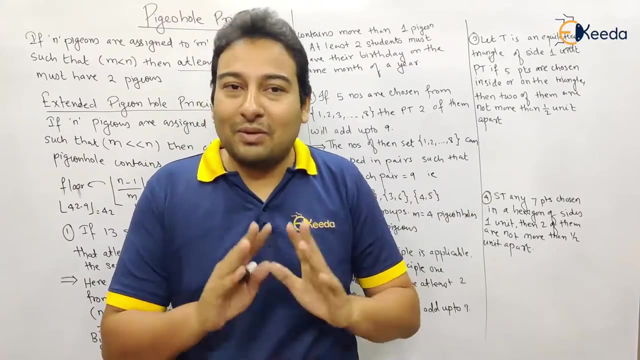 From a class Prove that at least two of them will have their birthday on the same day of a week. So eight students means what? N is equal to eight, Eight pigeons And M is equal to seven, That is, seven pigeonholes. M is less than N, Pigeonhole principle is applicable. That's it, Story over. 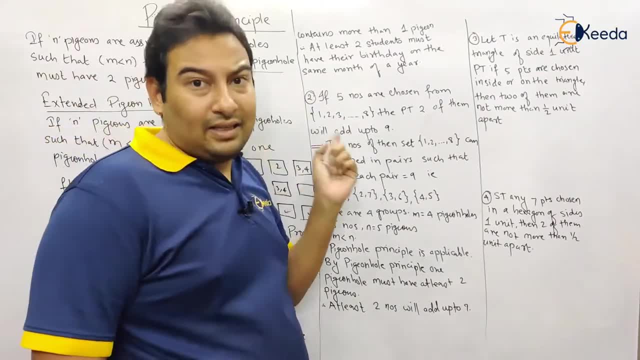 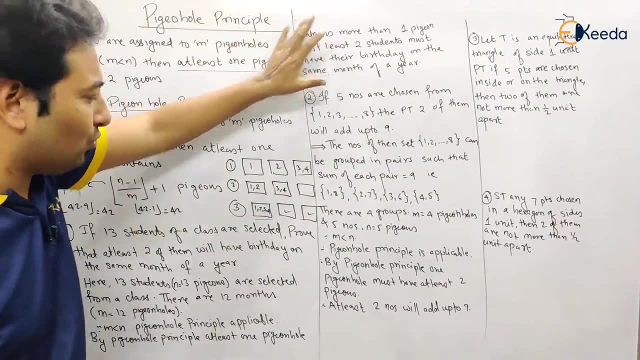 Next question. Now, this problem is a very important problem. It is asked a number of times in the exam. If five numbers are chosen from- and see, we have written the solution also, So you need to write it down in this particular format. If five numbers are chosen from one to: 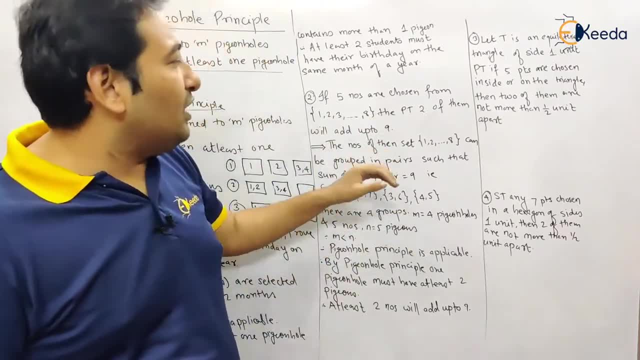 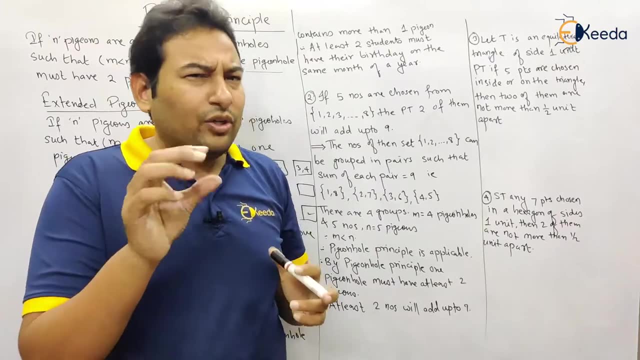 eight. So between one to eight, five numbers are chosen. We need to prove that two of them will add up to nine. We need to prove that two of them will add up to nine. So you need to remember, in this particular problem, See, two of them will add up to nine. So two numbers adding up to nine. So between one to eight, which two numbers will add up to nine. The first pair is 1,8. That will add up to nine. If you add, you will get nine, 2,7,, 3,6, and 4,5.. So these are the possibilities. If you add, you will. 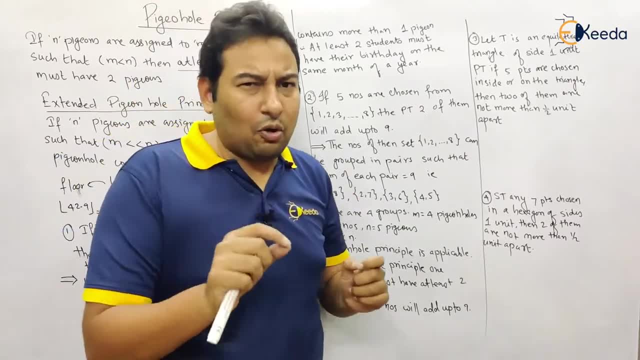 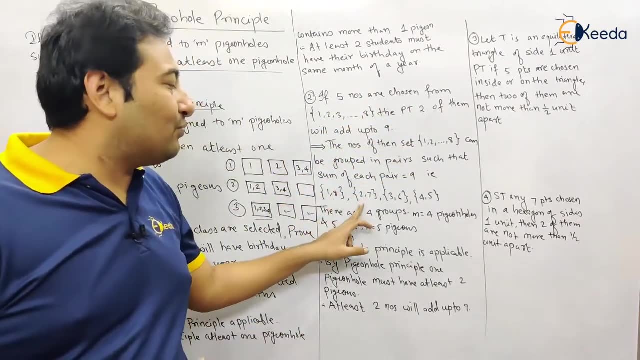 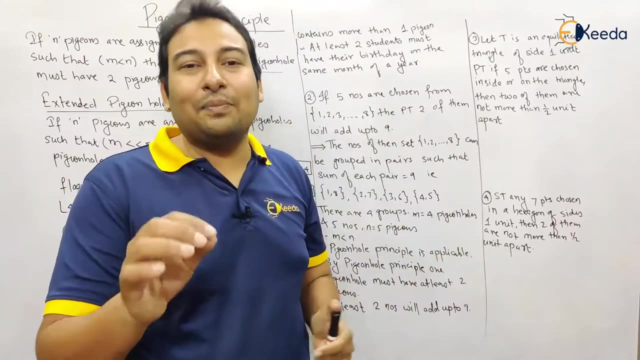 get the sum as nine. So you need to remember this. in this problem There is this trick you need to remember. So that's it Story over. Five numbers are chosen And how many sets. we are getting Four. So five numbers, That means N is equal to five pigeons. Four sets, That means M is equal. 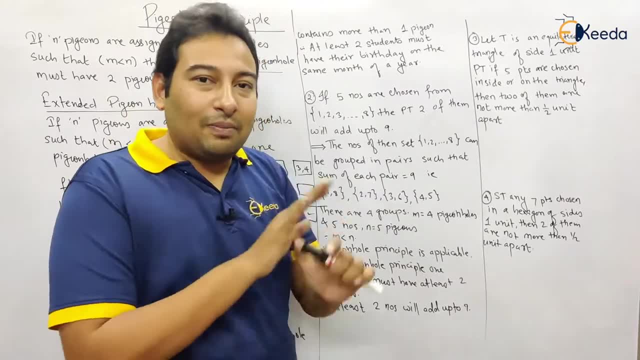 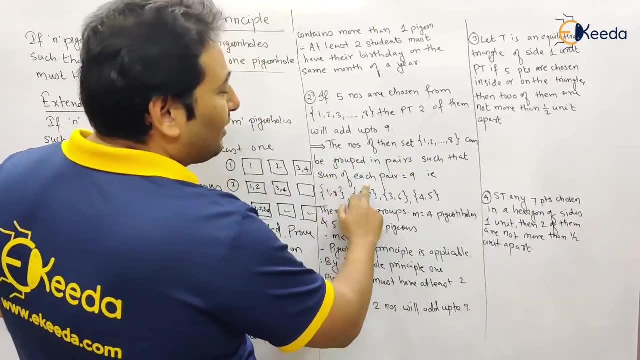 to four pigeonholes, M is less than N. Pigeonhole principle applicable Story over. Let me read the question for you. The number of sets can be grouped in pairs such that the sum of each pair is equal to nine. So these are the possibilities. There are four groups, So M is equal to four. 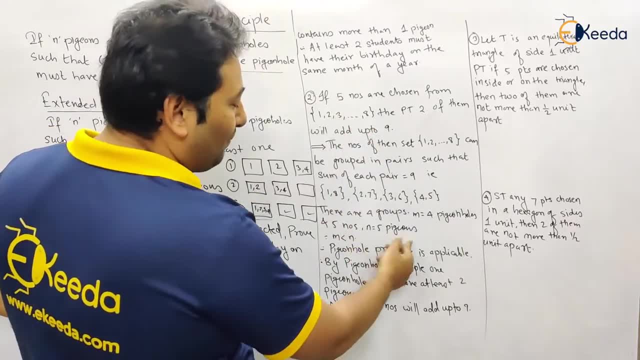 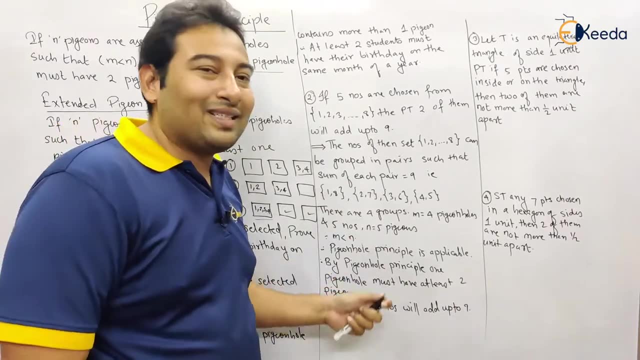 pigeonholes And five numbers are chosen. That means N is equal to five pigeons, M is less than N. Pigeonhole principle is applicable. Therefore, by pigeonhole principle, at least one of the pigeonhole must contain two pigeons. Therefore at least two numbers will add up to nine. So 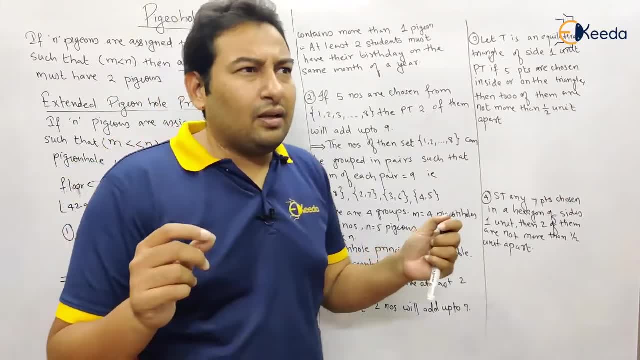 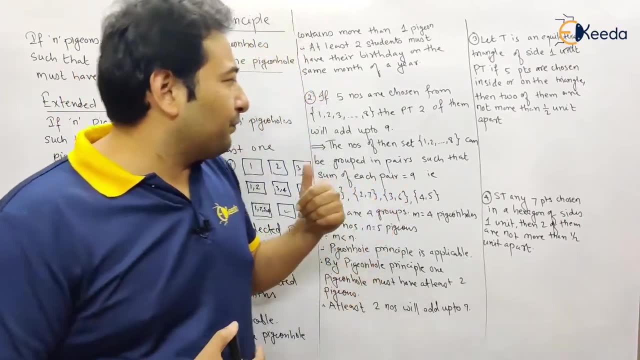 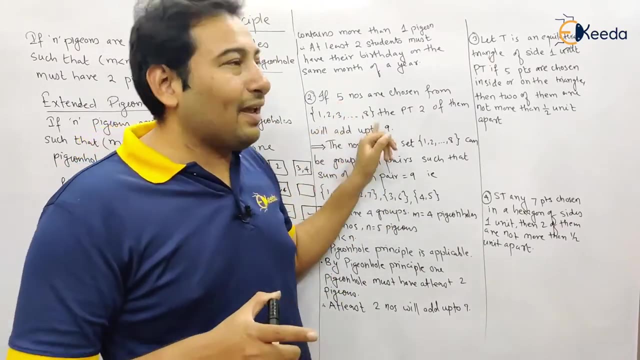 this is, you can say, a bit tricky problem, A bit difficult to digest, But yes, you need to remember the procedure. What is the next variation? One more variation has come in the exam And here it was seven numbers And here it is from one to eleven. So see here one comma, eight is nine. So it was the question. 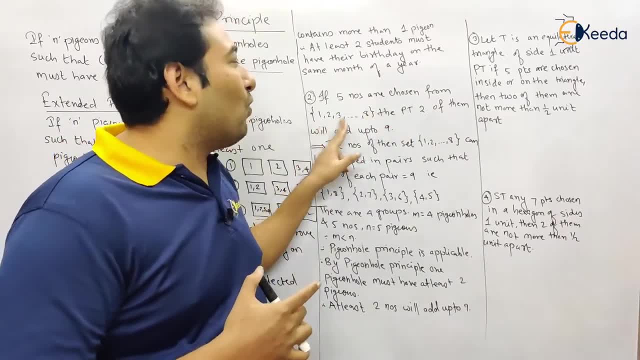 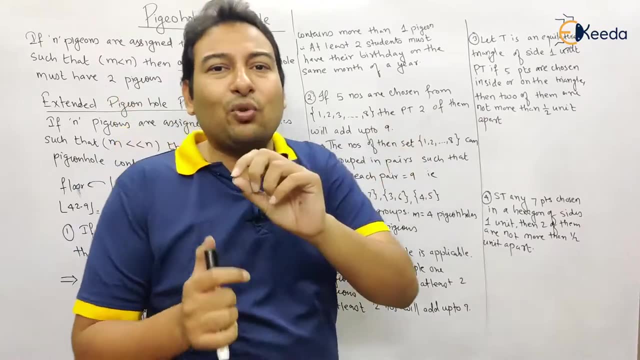 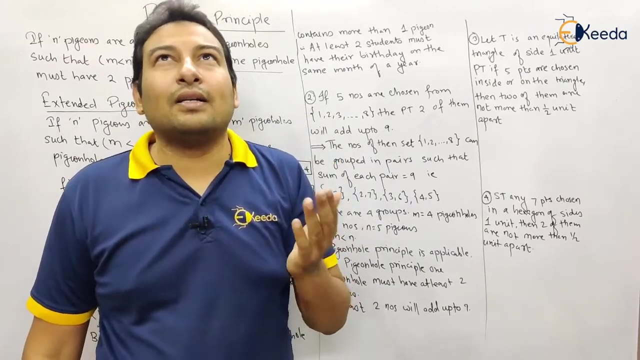 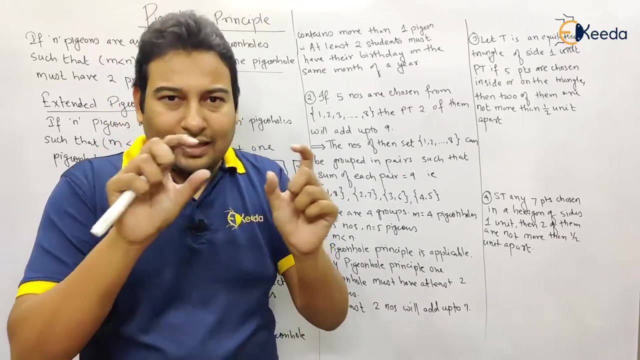 was something like this: Seven numbers are chosen from the set, one to eleven. Prove that two of them will add up to twelve, Because the first number is one and the last number is eleven. So you need to consider the pairs. So there are six pairs and seven numbers are chosen. So accordingly, 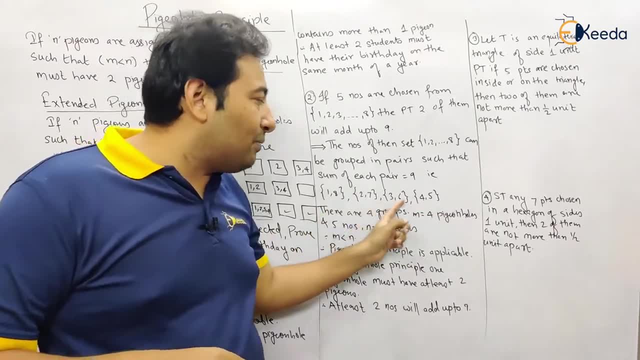 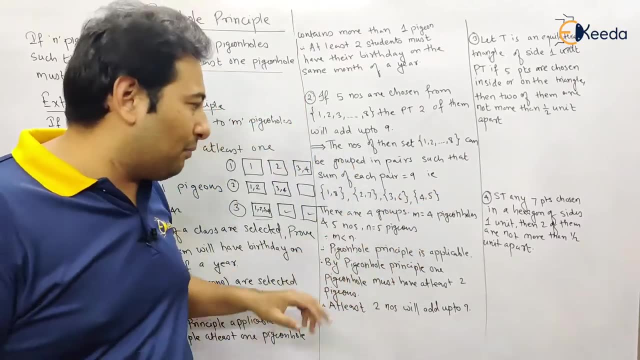 2 comma 7, 3 comma 6 and 4 comma 5. so these are the possibilities. if you add, you will get, get the sum as 9. so you need to remember this. in this problem there is a this trick you need to remember. so that's a story over five numbers are chosen and how many sets we are getting. 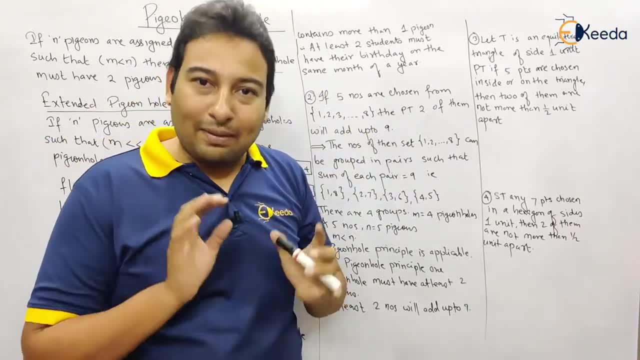 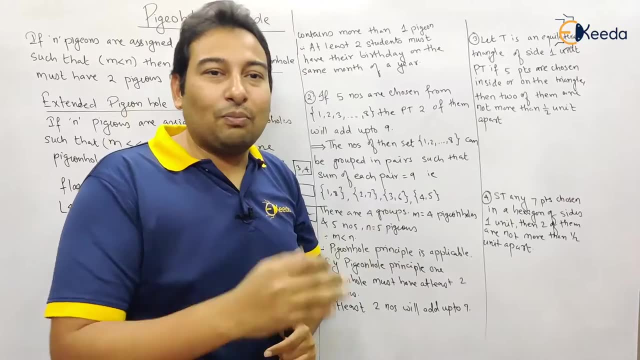 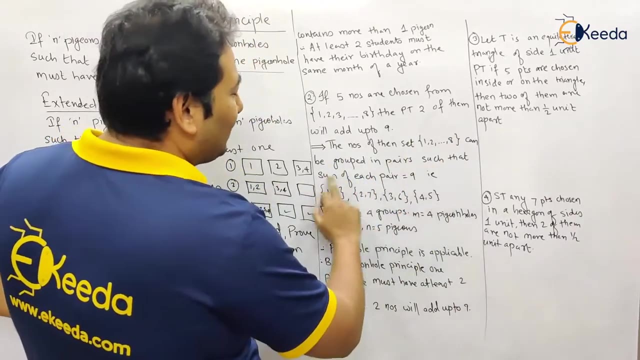 four, so five numbers. that means n is equal to five pigeons. four sets: that means m is equal to four pigeonholes. m is less than n. pigeonhole principle applicable story over. let me read the solution for you. the number of sets can be grouped in pairs such that the sum of each pair 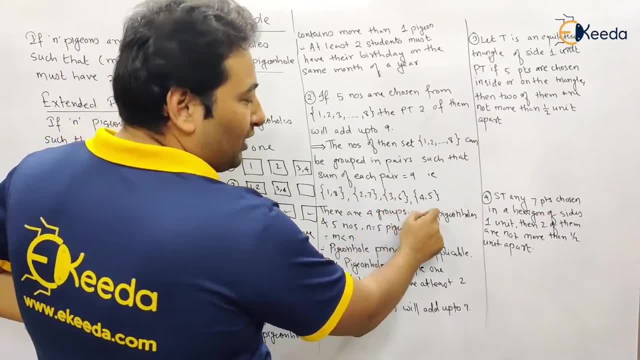 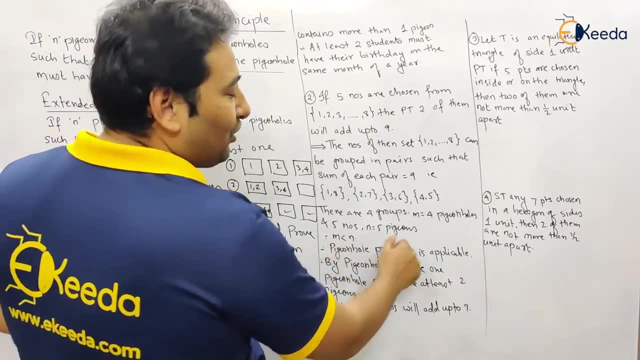 is equal to nine. so these are the possibilities. there are four groups, so n is, m is equal to four pigeonholes and five numbers are chosen. that means n is equal to five pigeons, m is less than n. pigeonhole principle is applicable, therefore, by pigeonhole principle, at least one of the pigeonhole 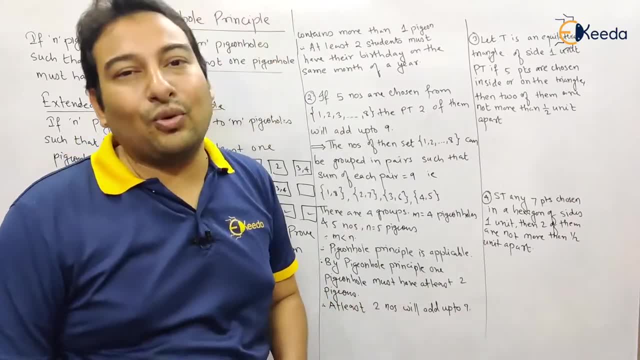 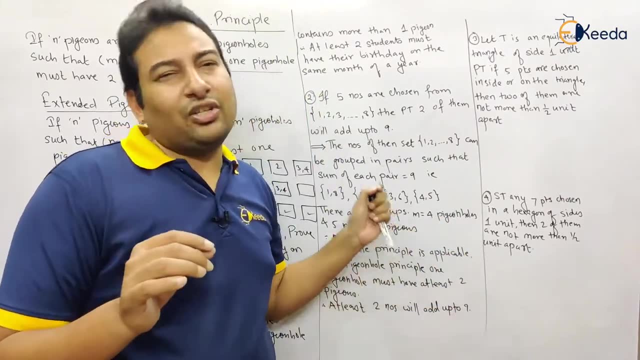 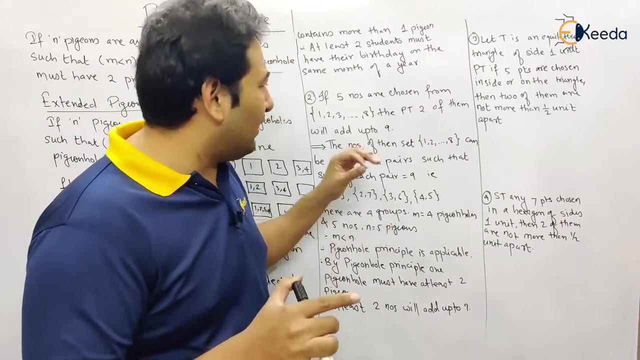 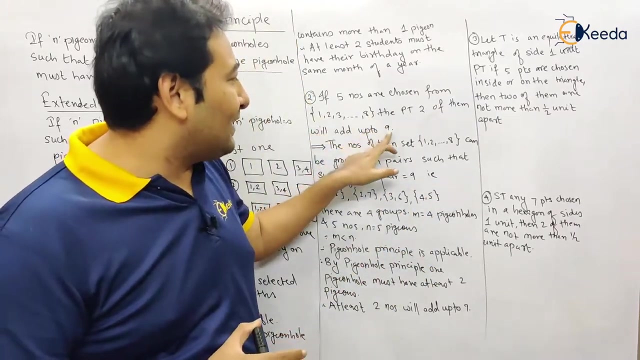 must contain two pigeons. therefore, at least two numbers will add up to nine. so this is you can. it is a bit difficult to digest but yes, you need to remember the procedure. what is the next variation? one of one more variation has come in the exam, and here it was seven numbers and here it is from 1 to 11. so see here, 1 comma 8 is 9, so it was. 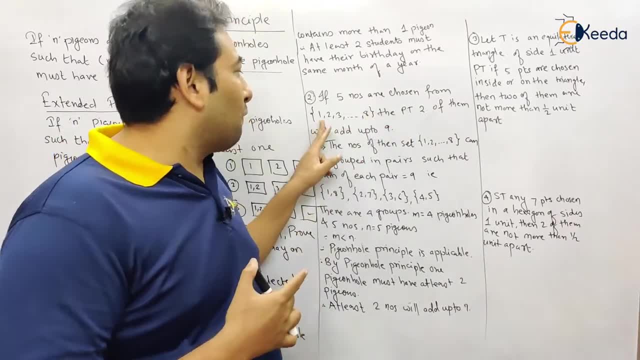 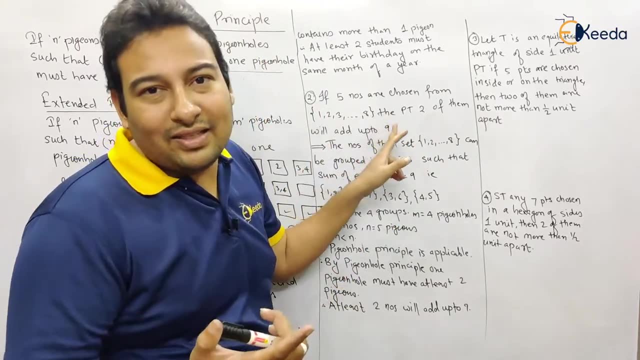 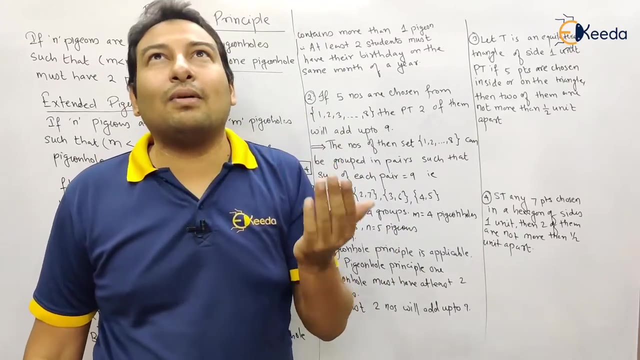 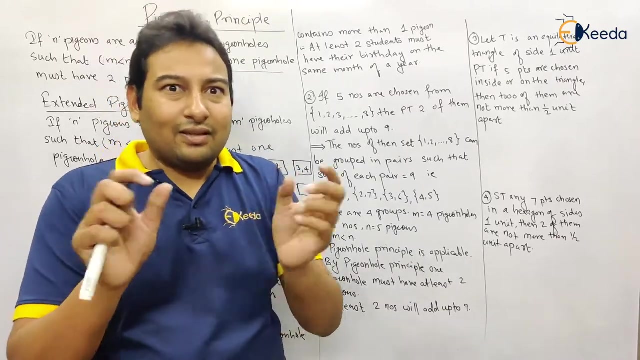 the question was something like this: seven numbers are chosen from the set 1 to 11. prove that two of them will add up to 12, because the first number is 1 and the last number is 11. so you need to make one comma 11, 2 comma 10, 3 comma 9, 4 comma 8, 5 comma 7, and that's it. so just consider the pairs. so. 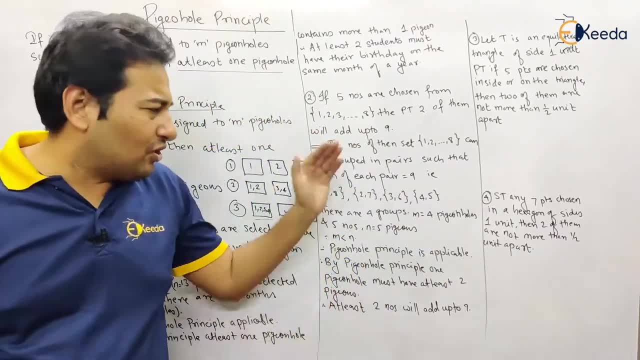 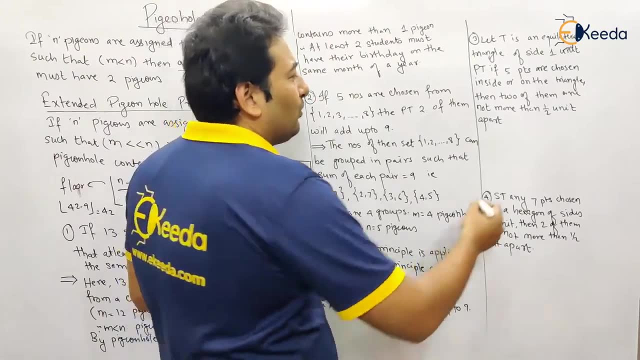 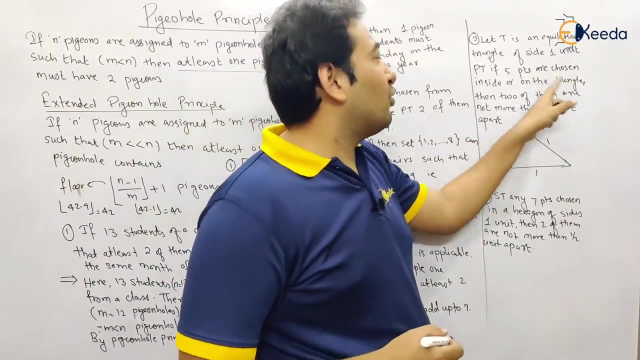 there are six pairs and seven numbers are chosen. so accordingly- pigeonhole principle- you will get your solution. next problem: let t is an equilateral triangle of side one unit. so it's an equilateral triangle of side one unit, so that if five points are chosen inside or on the triangle, so we need to choose five points. 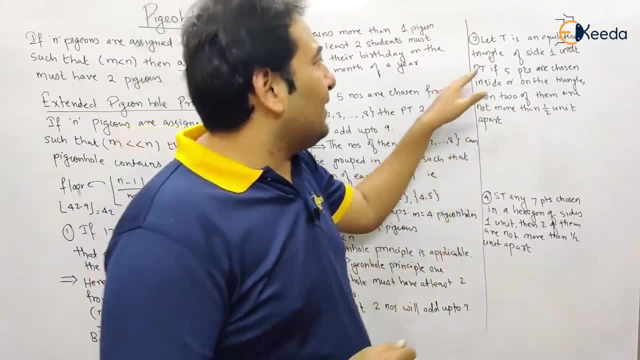 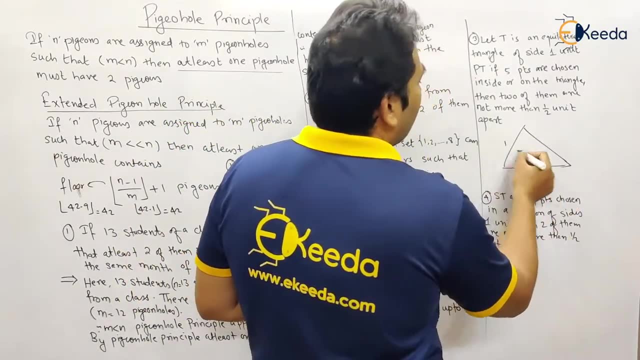 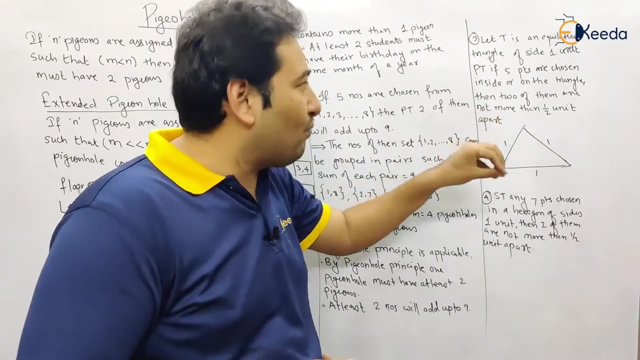 pigeonhole principle: you'll get your solution. Next problem: Let T is an equilateral triangle of side one unit. So it's an equilateral triangle of side one unit. Prove that If five points are chosen inside or on the triangle, So we need to choose five points, Then two of 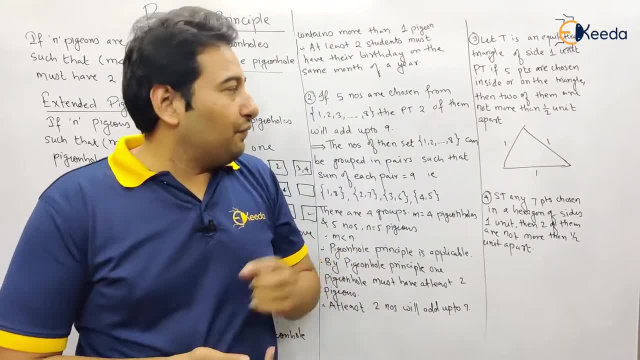 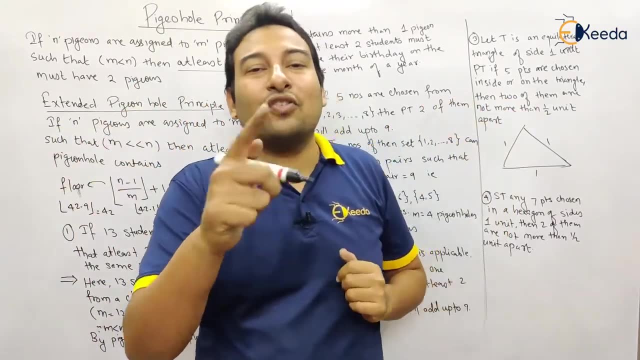 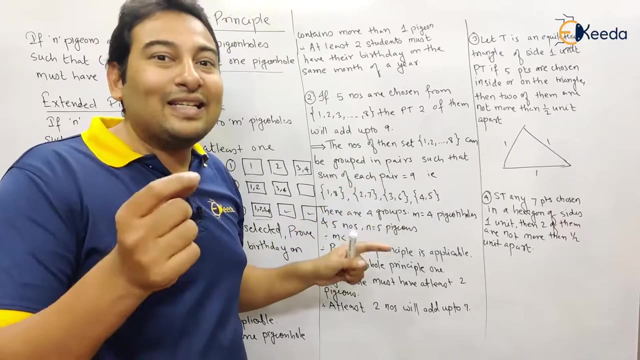 them are not more than half unit apart. We need to choose five points. See, it's very simple. again, See any. if you observe all this problem, there is a difference of one. See here there were 13 students, twelve months. Next problem: There are four sets, five numbers. There is a difference of. 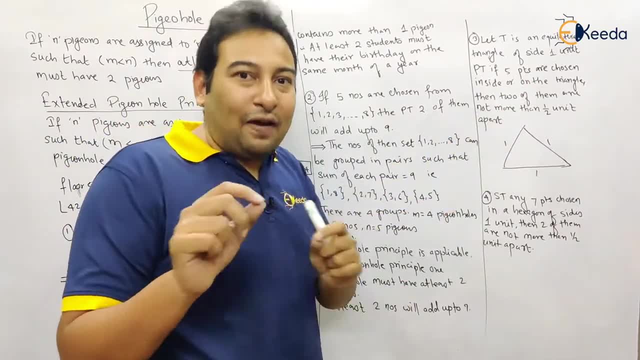 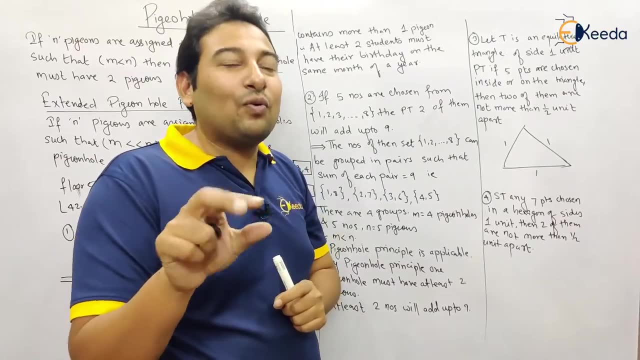 one. Here we need to choose five points, So any of five points. that means n is equal to one. So n is equal to five. That is five pigeons. So m will be less than one. That is what four. So anyhow. 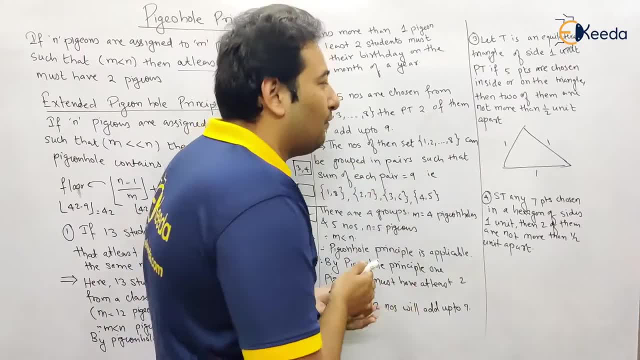 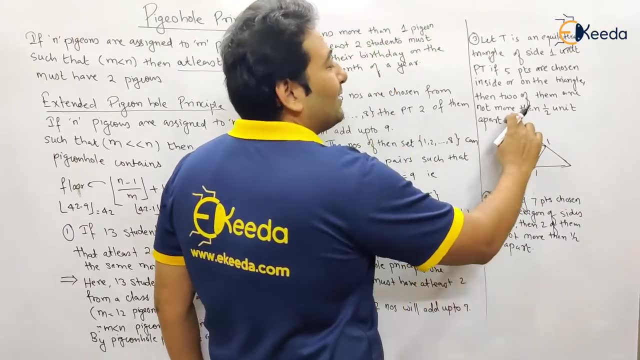 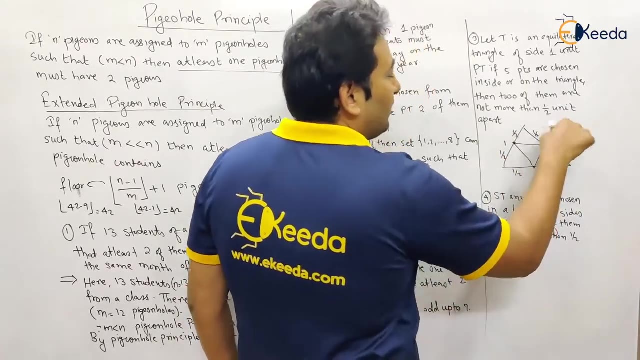 we need to divide this triangle into four regions. How? See here, Let me take the midpoint and let me join these midpoints. Why? Because it is written half unit Now. since it is a midpoint, every this is length of half unit. Now, if you choose any point, so where the point will belong. 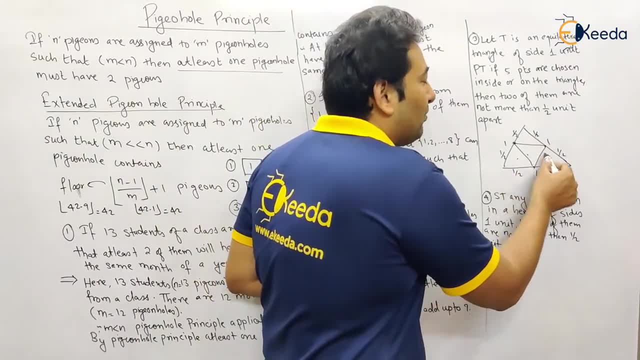 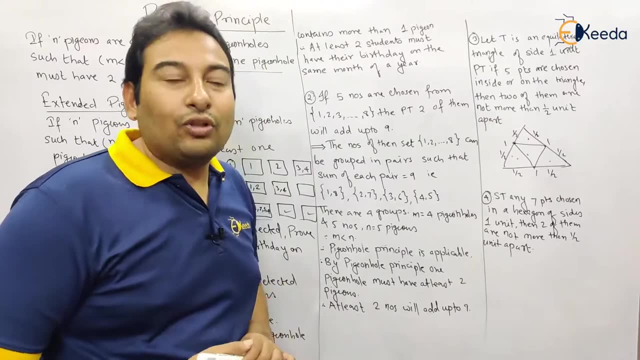 five points where it can be at the extreme possibilities. They all are from the different region, but at least there will be a region in which more than more than one point, or you can say simply two points. So story is over. Five points are chosen, So five points are chosen. 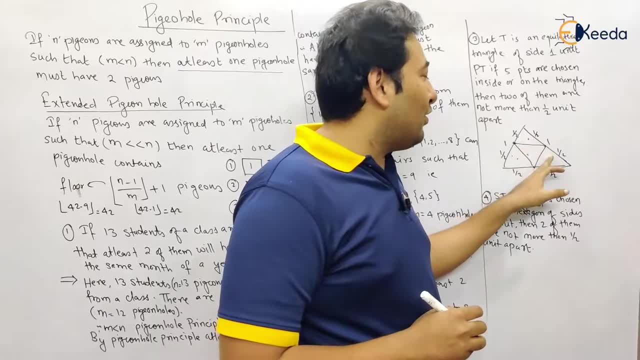 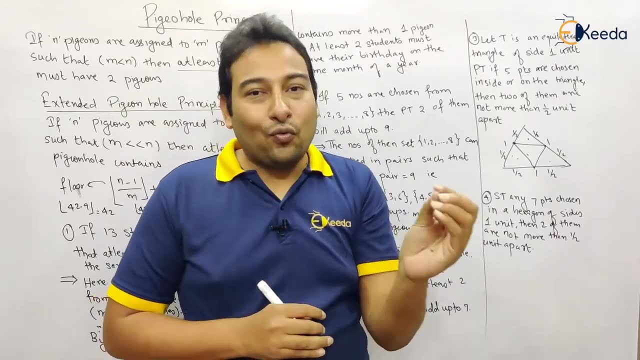 n is equal to five, That is pigeons. And how many regions are there? One, two, three, four. So five points is equal to n is equal to five. is number of pigeons M is equal to four. number of pigeons M is less than n. Pigeonhole principle is applicable. According to pigeonhole principle. 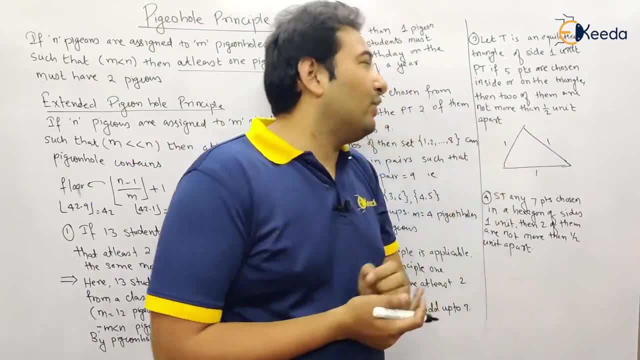 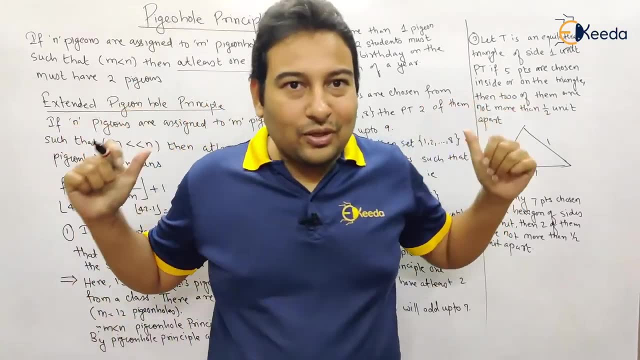 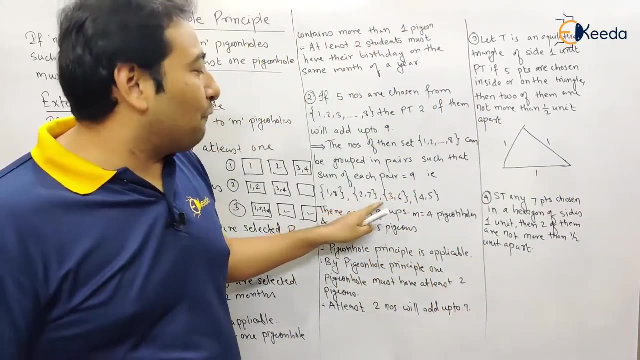 then two of them are not more than half unit apart. we need to choose five points. see, it's very simple. again, see any. if you observe all this problem, there is a difference of one. see, here there were 13 students, 12 months. next problem: there are four sets, five numbers. there is a difference of one. 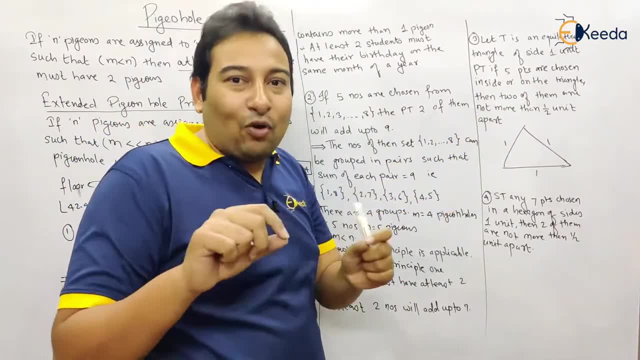 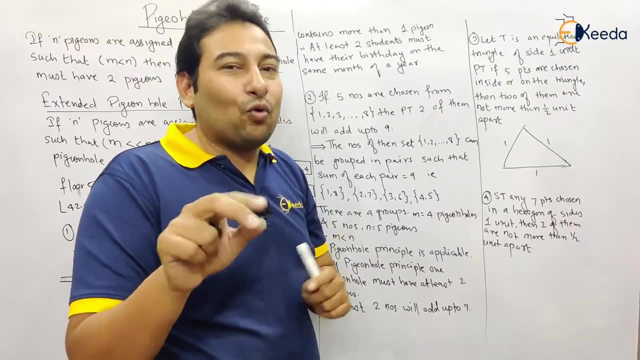 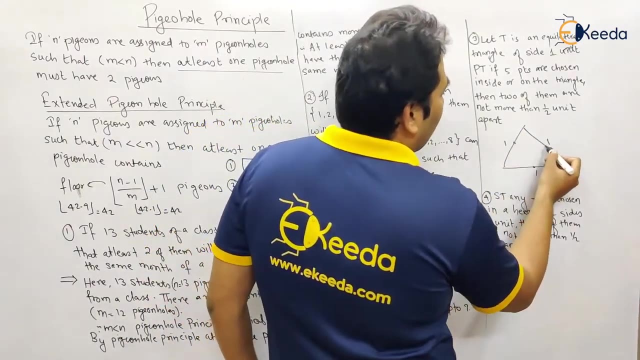 here we need to choose five points, so any of five points, that means any of the five points is equal to five. that is, five pigeons, so m will be less than one. that is what four, so any of. we need to divide this triangle into four regions. how see? here, let me take the midpoint and let me join these. 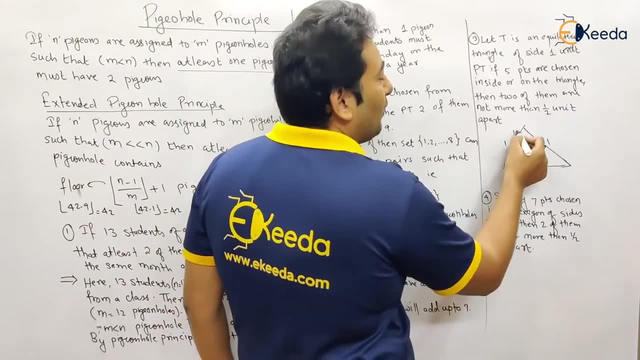 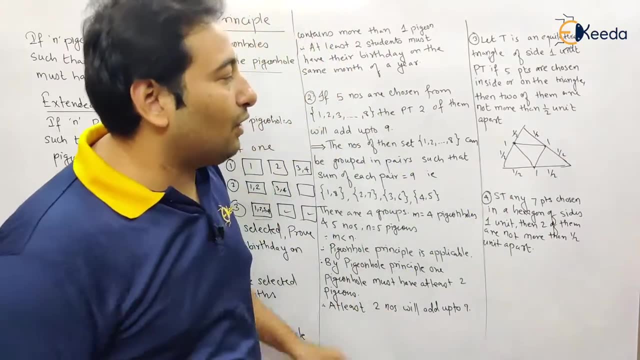 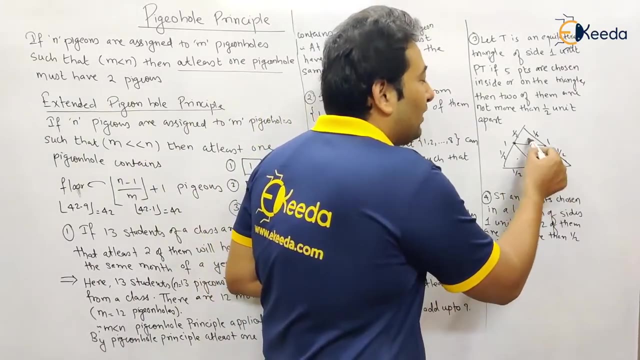 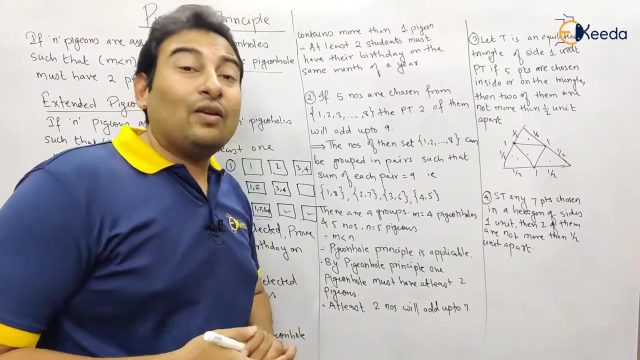 midpoints. why? because it is written half unit. now, since it is a midpoint, every this is length of half unit. now, if you choose any point, so where the point will belong, five points where it can be at the extreme possibilities. they all are from the different region, but at least there will be region in which more than more than one point, or you can say: 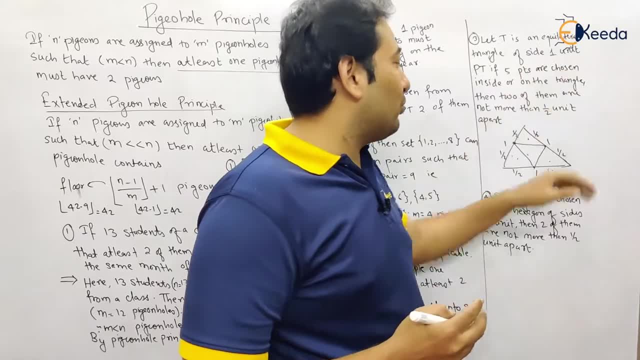 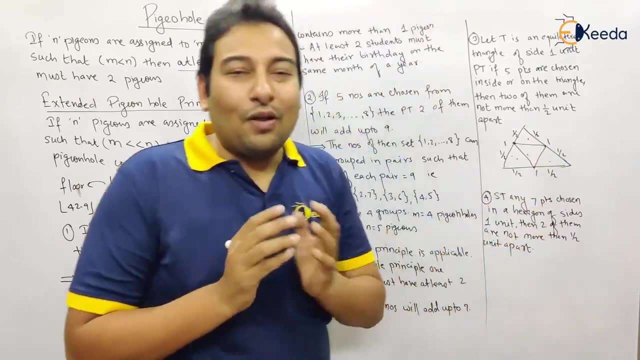 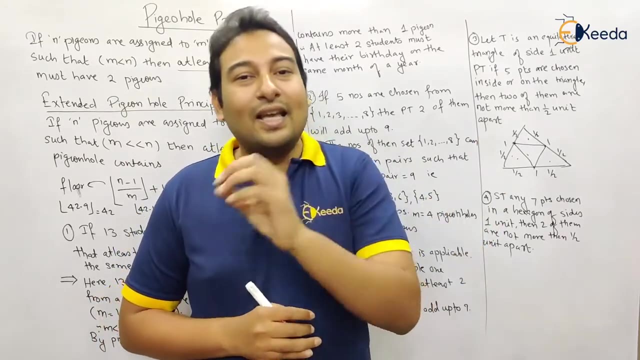 simply two points. so story is over. five points are chosen. so five points are chosen. n is equal to five, that is pigeons. and how many regions are there? one, two, three, four. so five points is equal to. n is equal to five. is number of pigeons: m is equal to four. number of pigeon holes: m is. 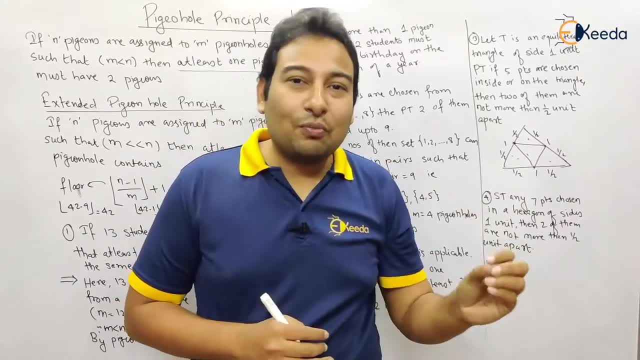 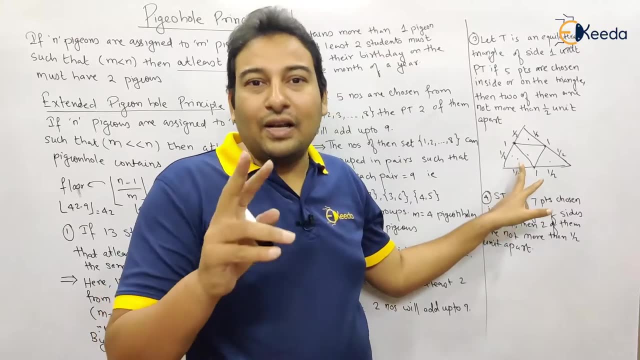 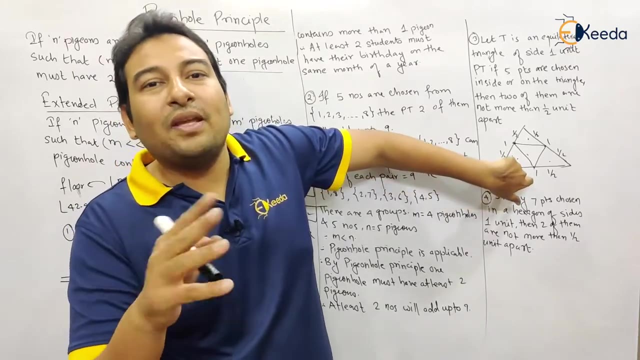 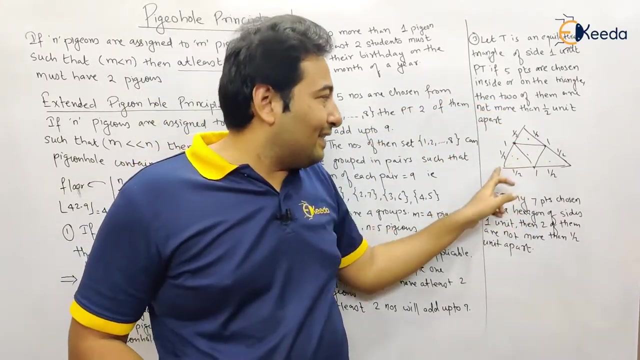 less than n region hole principle is applicable. according to vision or principle, at least one pigeon hole must contain two pigeons. therefore, at least one region will contain two points. if one reason contains two points, obviously they cannot be more than half unit apart. see, this is half unit. this is half unit. this is half unit. if you choose points in this triangle, obviously they 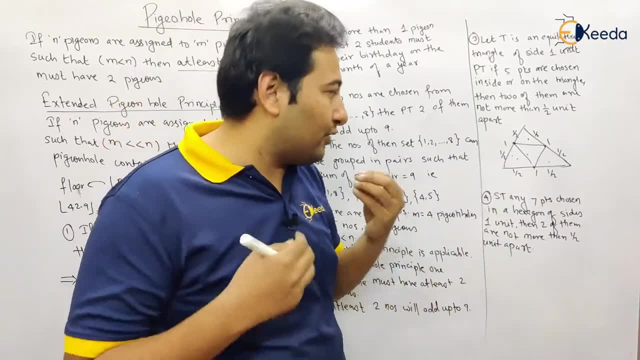 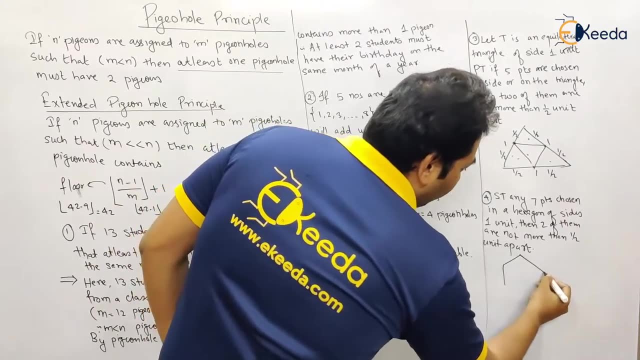 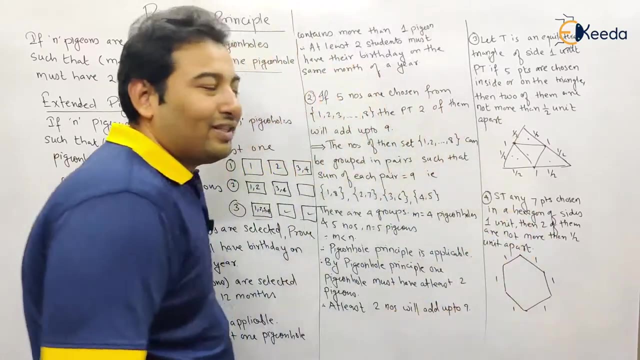 can be not more than half unit apart, so this is the way you're going to write it on. the solution for this next show that any seven points are chosen in a hexagon. hexagon means six sides. seven points are chosen, so how many regions will be there? 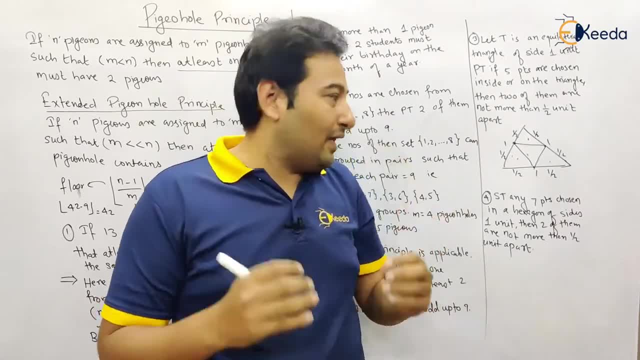 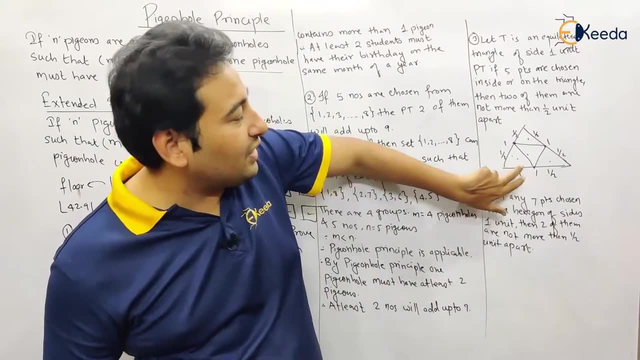 at least one pigeonhole must contain two pigeons. Therefore, at least one region will contain two points. At least one region will contain two points. If one region contains two points, obviously they cannot be more than half unit apart. See, this is half unit, This is half. 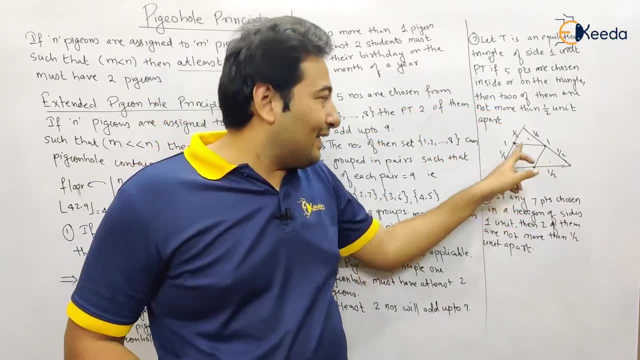 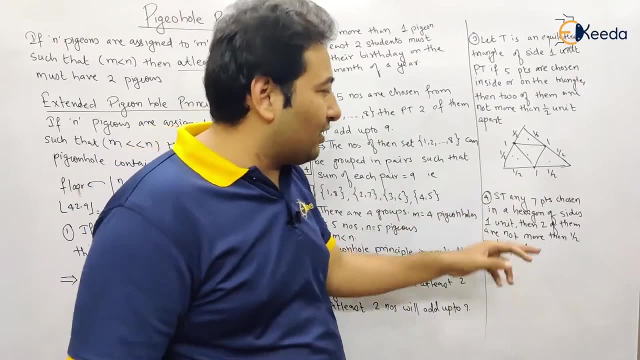 unit. This is half unit. If you choose points in this triangle, obviously they can be not more than half unit apart. So this is the way you're going to write it. So let's write down the solution for this. Next, show that any seven points are chosen. 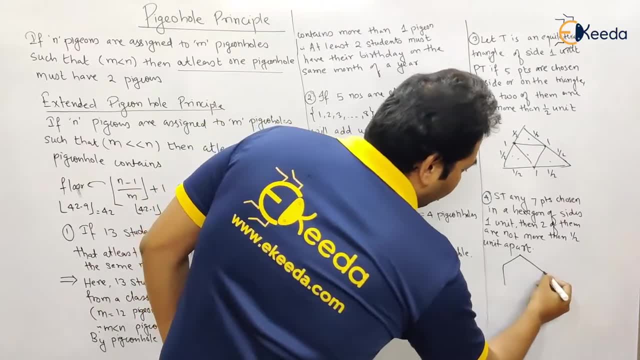 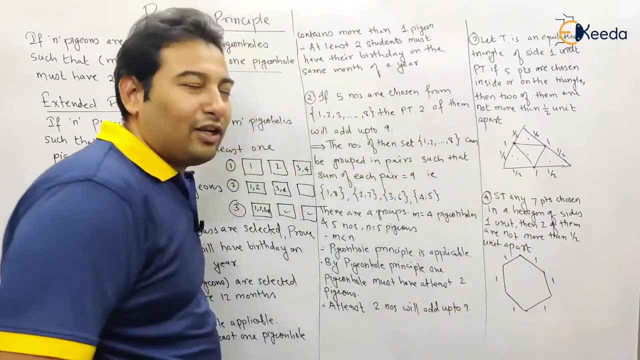 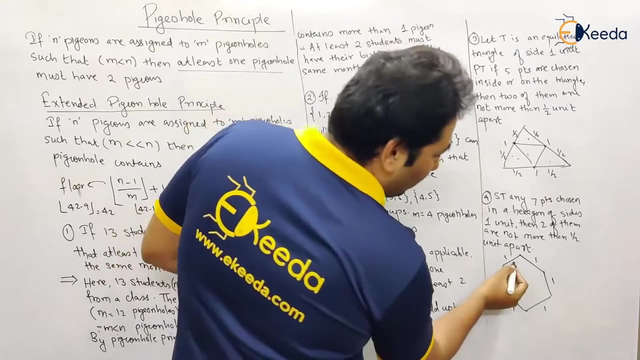 in a hexagon. Hexagon means six sides. Seven points are chosen. So how many regions will be there? Six regions In all the possibilities. there is a difference of one between pigeon and pigeonholes, So let me first find it out. It's midpoint. 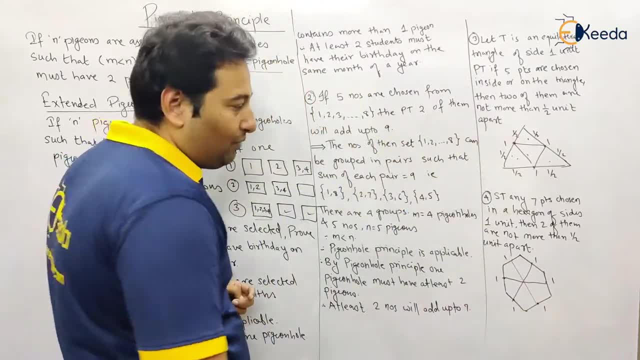 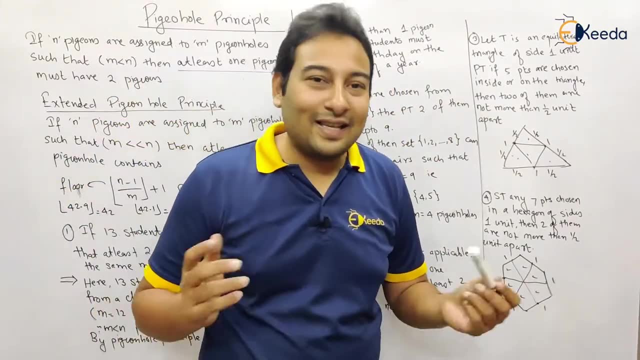 See here How many regions we have: One, two, three, four, five, six. Story over Seven points: N is equal to seven pigeons, M is equal to six pigeonholes, M is less than n, So therefore, 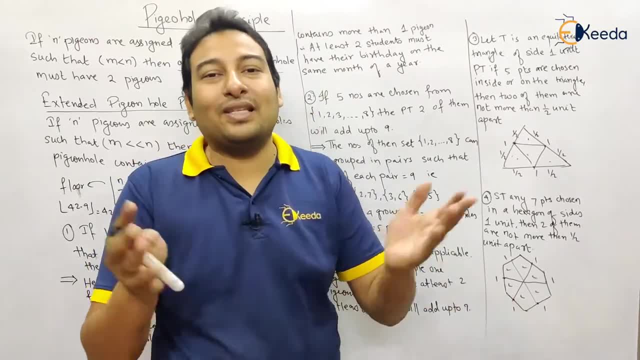 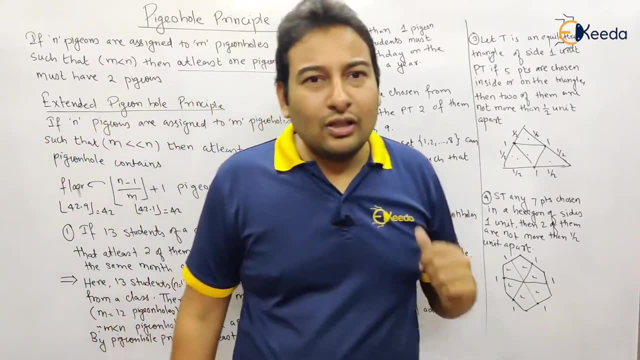 at least one region will contain two points, So obviously they are not more than half unit apart. That's it Story over. So that is what pigeonhole principle is In all the problems there is a difference of one, Or you can simply say: if there is a small difference. 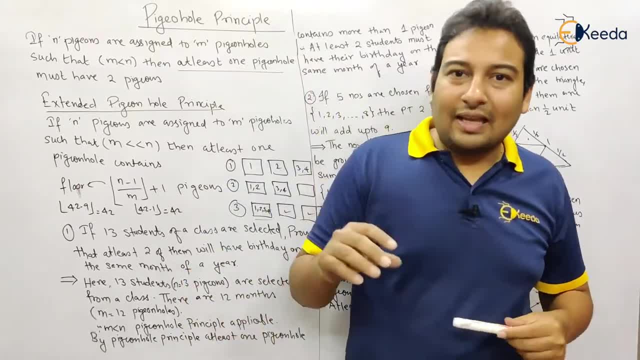 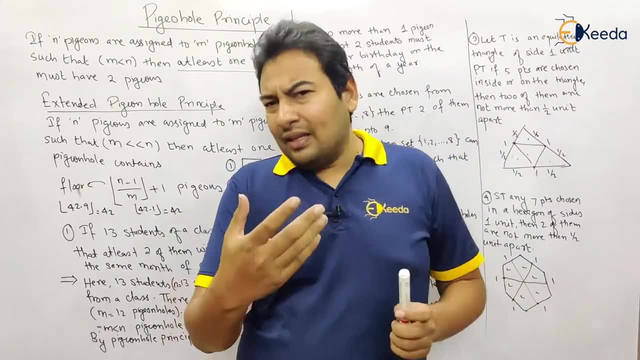 you can directly write it on by using pigeonhole principle. If there is a big difference, then you're going to go ahead with the formula extended pigeonhole principle. But yeah, in all the problems you can apply this formula, You'll always get the same result. Let's talk. 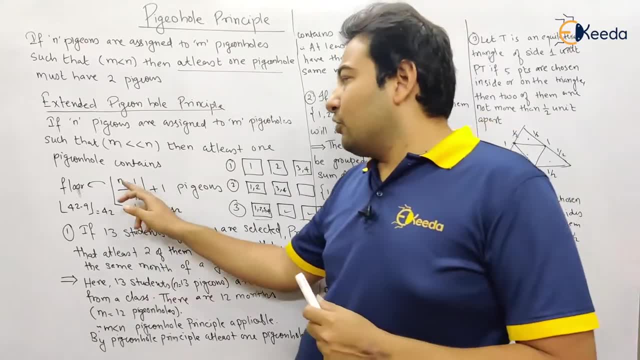 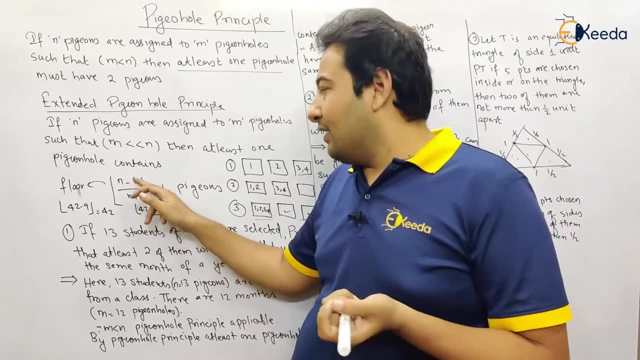 about this. How many students are there? 13 students of a class, So n is 13 and 12 months. So this is what 13 minus 1, 12.. 12 divided by 12.. So 12 divided by 12 is what 1.. So floor of 1 is: 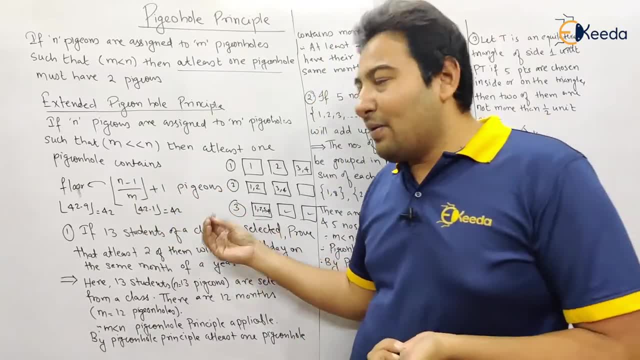 1. 1 plus 1 is what? 2.. So at the end of the day, you can write it down. So you can write it down At least one month in which two students born. So you can always apply this formula, But for a. 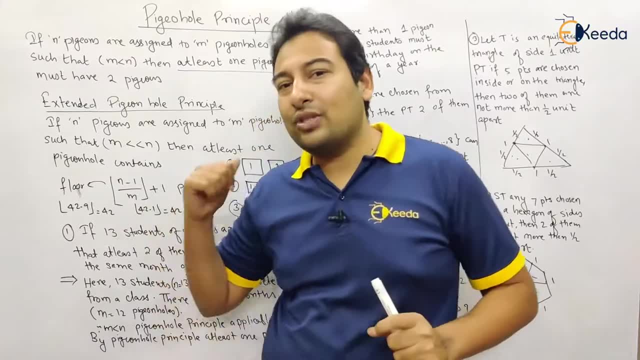 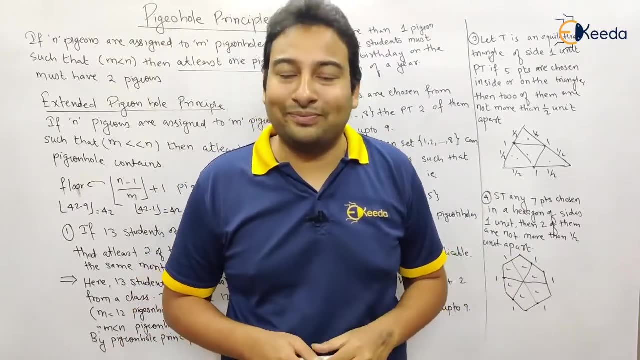 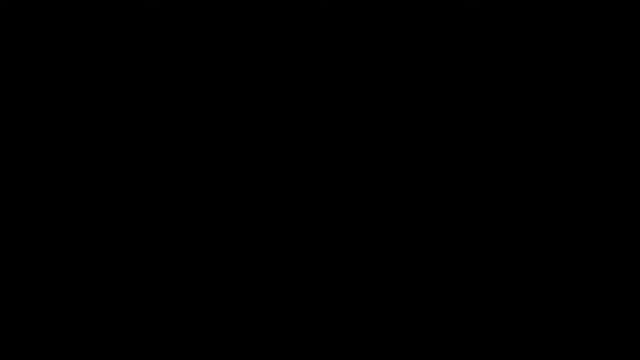 small numbers. we don't apply the formula for a big difference. We use extended pigeonhole principle. So that's it for this video. In the next video, we'll talk about extended pigeonhole principle. Thank you for watching this video. Thank you for watching this video. 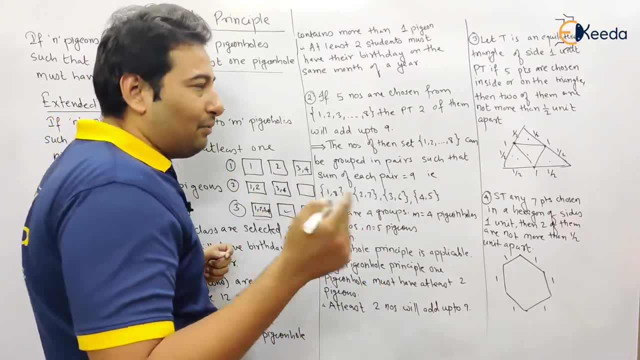 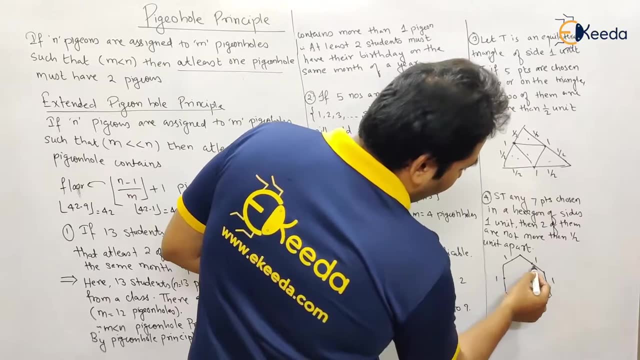 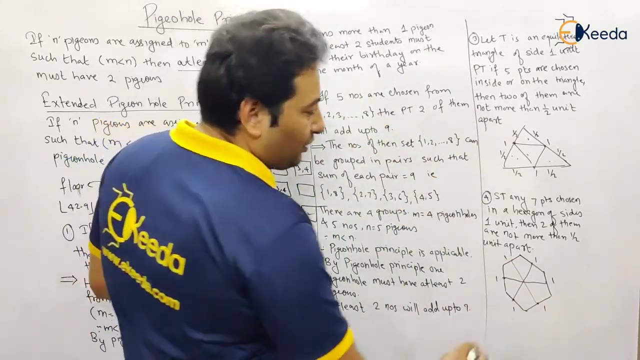 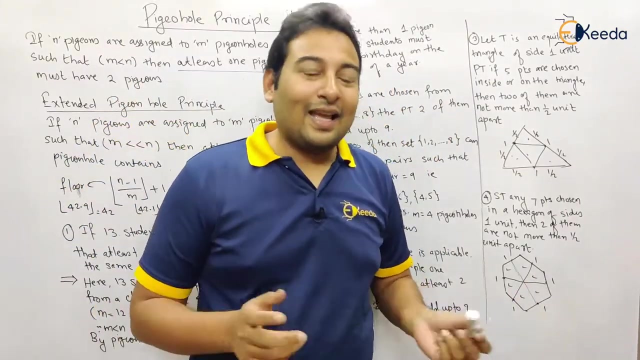 six regions. in all the possibilities, there is a difference of one between pigeon and pigeon holes, so let me first find it out its midpoint. see here how many regions we have: one, two, three, four, five, six. story over seven points: n is equal to seven pigeons. m is equal to six pigeon holes. m is less than. 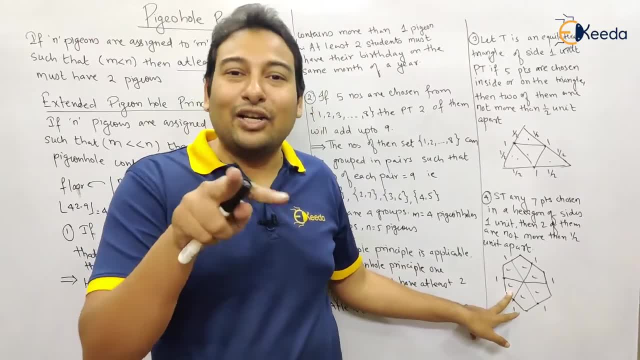 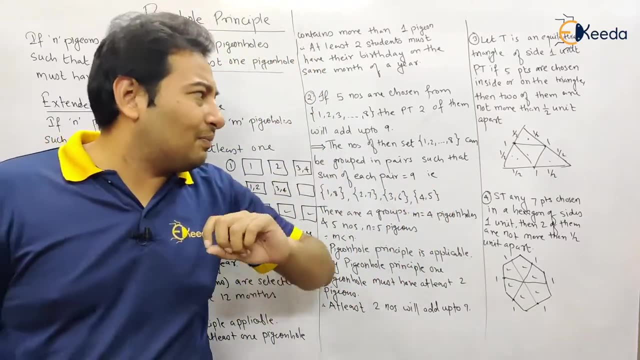 n. so therefore at least at least one region will contain two points, so obviously they are not more than half unit apart. that's it story over. so that is what pigeon hole principle is in all the problem. there is a difference of one, or you can simply say: if there is a small difference, you can. 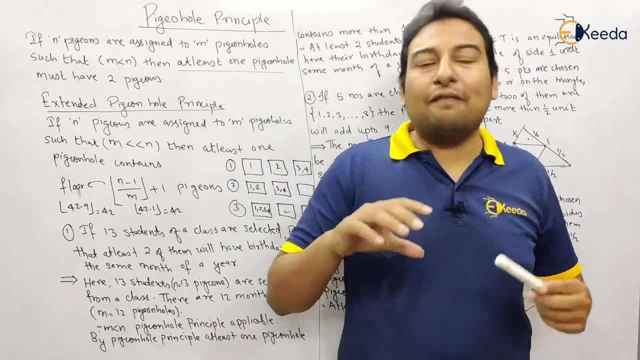 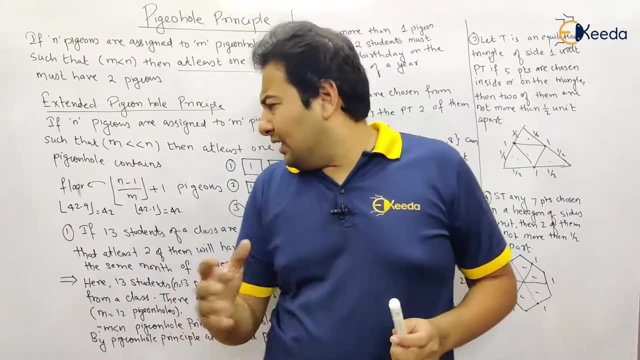 directly say that there is a difference of one, or you can directly say that, write it on by using pigeonhole principle. if there is a big difference, then you're going to go ahead with the formula extended pigeonhole principle. but yeah, in all the problems you can apply this formula. you will always get the 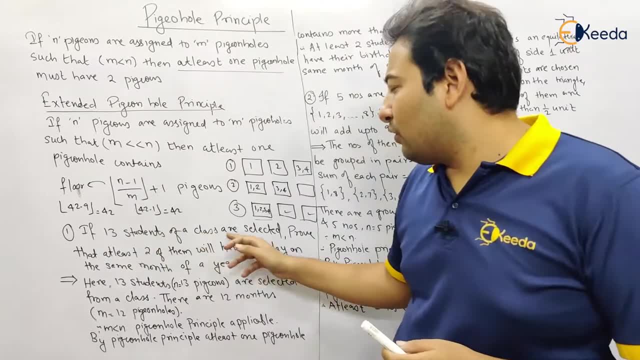 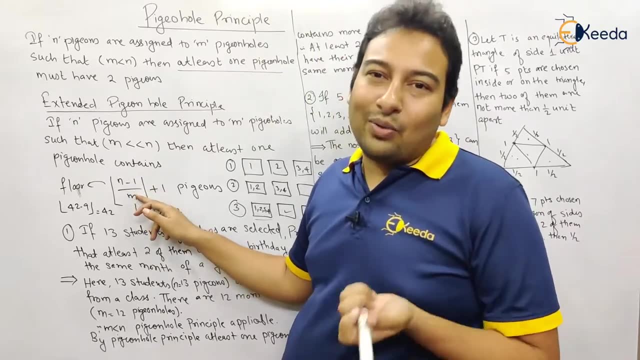 same result. let's talk about this. how many students are there? 13 students of a class, so n is 13 and 12 months. so this is what 13 minus 1, 12, 12 divided by 12. so 12 divided by 12 is what 1. so floor of 1 is 1. 1 plus 1 is what 2. so at least. 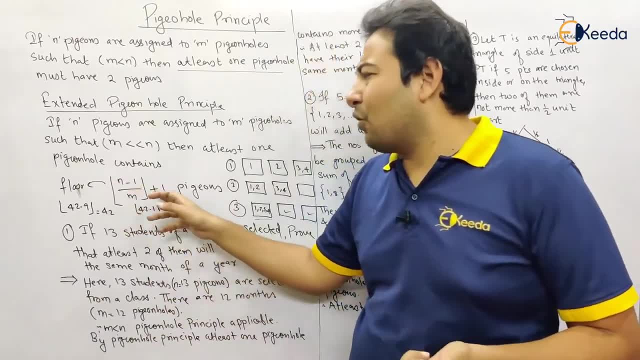 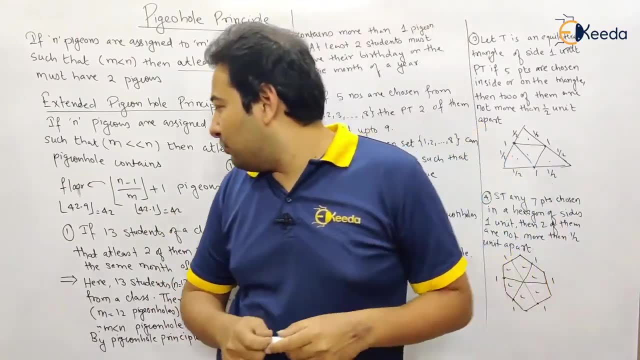 1 month in which 2 students born. so you can always apply this formula, but for a small numbers we don't apply the formula. for a big difference, we use extended pigeonhole principle. so that's it for this video. in the next video we will talk about extended pigeonhole principle. thank you for watching this video. you.